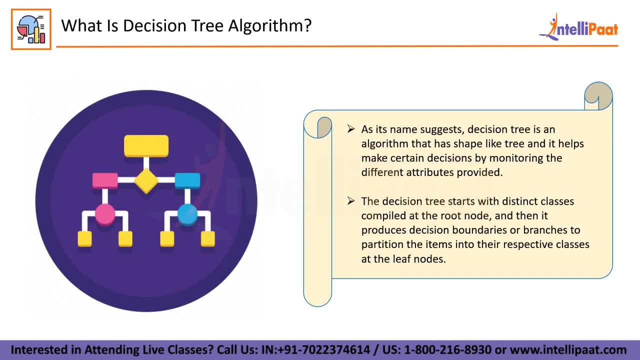 you guys can gauge what it really stands for from its nomenclature itself. It's something like a tree used to make some sort of decisions, Whether it is classification or regression. you can see that there is a degree of correlation between the data features we get And by leveraging. 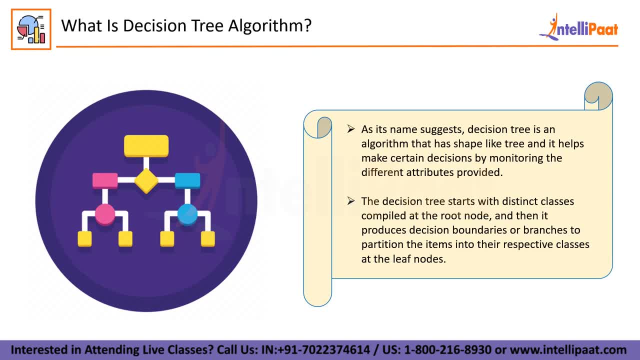 the same, we are able to build a pattern and predict the future outcomes. Decision Tree Algorithm is completely built around this fact itself. Decision trees create a tree-like structure by comprehending the relationship between features. It begins with different classes at the root node and then it creates decision boundaries or branches. 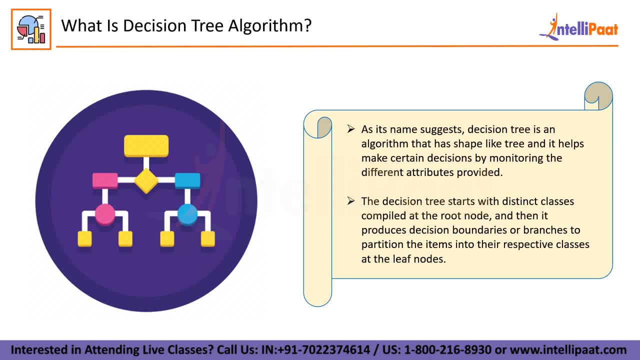 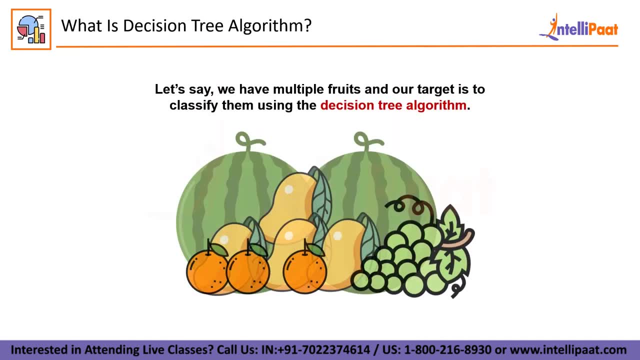 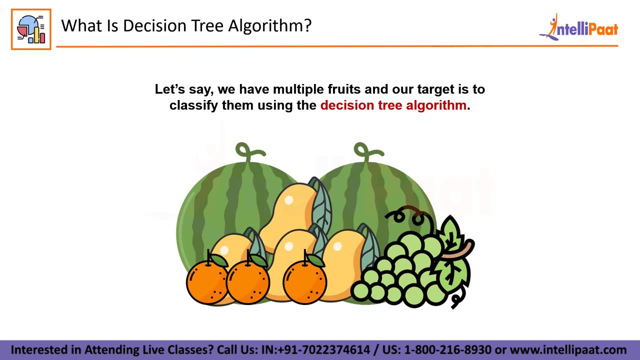 to split the items into their respective classes at the final leaf nodes. Let me give you a sample example of how this algorithm looks like. So let's say we have multiple fruits over here. Let's say we have multiple fruits over here here, brought fresh from the market, and we want to keep them inside the fridge by categorizing. 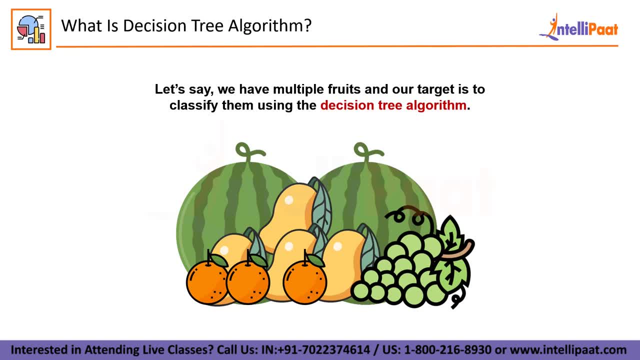 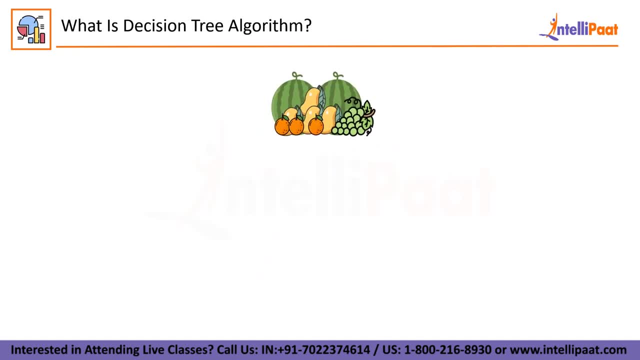 them into their different own categories. You can see that we have oranges, mangoes, watermelons and grapes over here, So initially all of this will be assumed at the root node. Then we'll put down the condition to split these fruits at the next level. Now let's 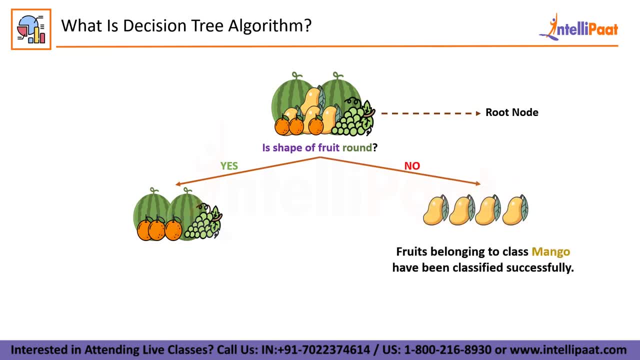 say, we'll check whether the shape of the fruit is round or not. If it is round, then it will go to the left side of the tree, and if it is not, then it will go to the right side of the tree. Now you can see that all the mangoes have been separated over here. 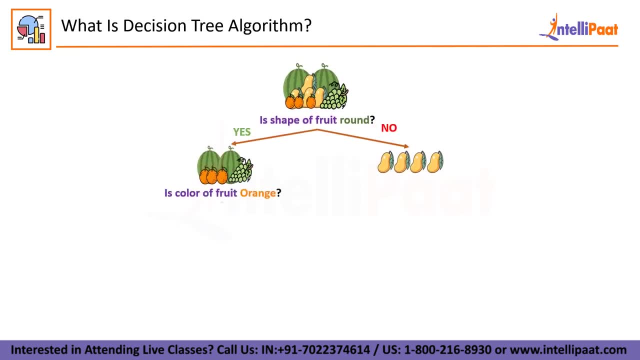 Next we'll just move ahead in the direction of the left node. Next condition will be to check whether the color is orange or not. With this condition we'll have oranges separated from the lot. Now. the next decision boundary we'll put across will be to check whether 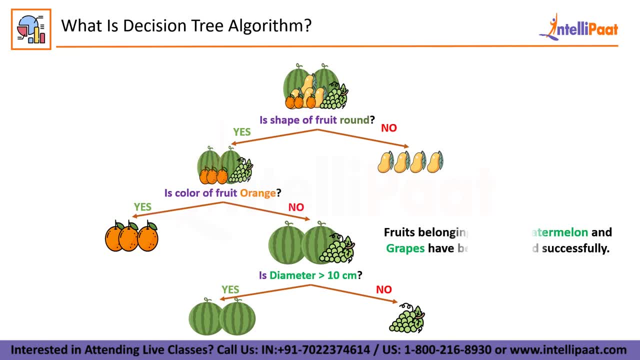 if the diameter is greater than 10 cm. If it is greater than 10 cm, the fruit will be watermelon and if not, the fruit will be grape. Now here you can observe that with each node after the root node, we're actually 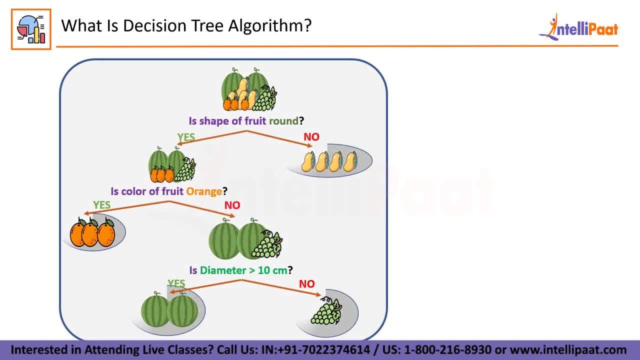 classifying the data into its labels successfully. The last nodes, such as this node representing oranges, watermelons, mangoes and grapes, are called as leaf nodes And- yes-no decision boundaries you see over here- are called as branches. Now, this was kind of a classification problem, but besides this, decision tree algorithm. 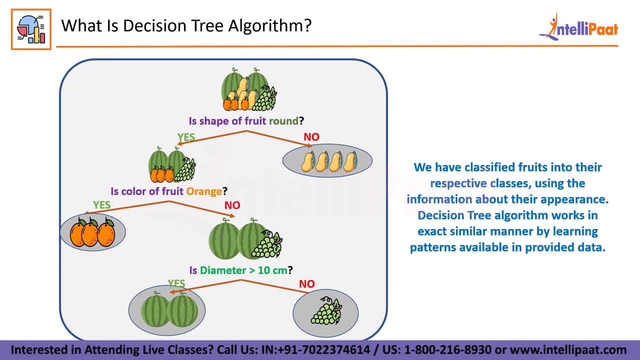 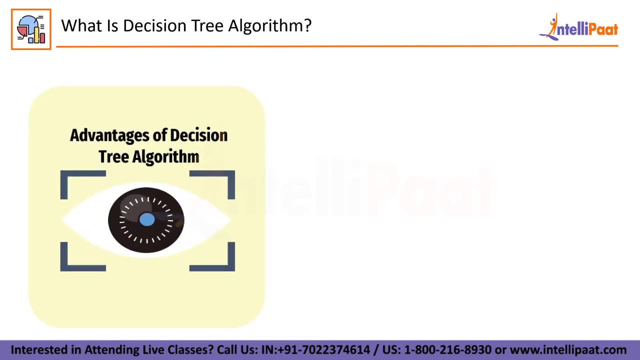 can also solve regression problem, Just in the conditions. there will be influence of numbers instead of classes. In case of regression, each decision is made based on the sum of squared error. That being said, let me tell you a few advantages of this algorithm. First, 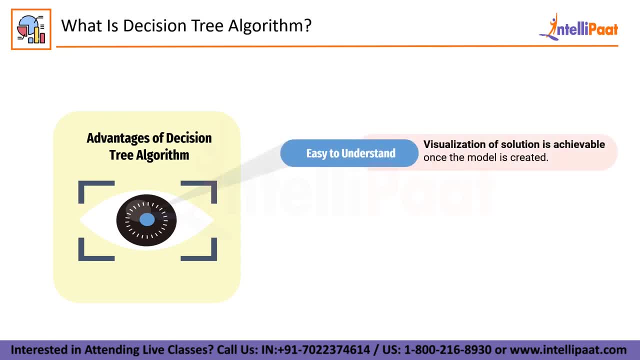 advantage we have here is that the decision tree algorithm is quite easy to understand, interpret and visualize. Once you create the model, by using decision tree classifier or decision tree regressor, you can visualize how the classification is achieved after processing your training data through the model, And this makes the visualization of classification 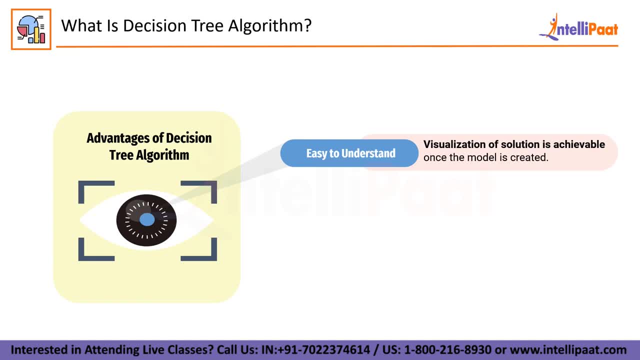 increasingly simple. We'll see that through our coding implementation part as well. Second advantage we have here is that there is no assumption that this algorithm makes about the data. It can work well with the both continuous as well as categorical data, which makes it a very special algorithm, That's. 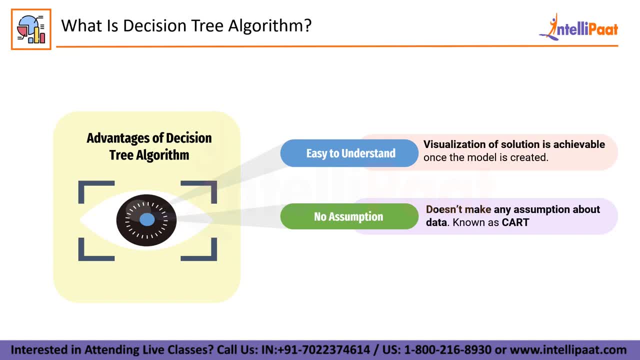 the sole reason why this algorithm is also termed as CART, or classification and regression tree. Next advantage of this algorithm is that its performance doesn't get affected by non-linear parameters. Now that we have learnt about the advantages, let me tell you about few limitations or disadvantages of this algorithm as well. First, we have to 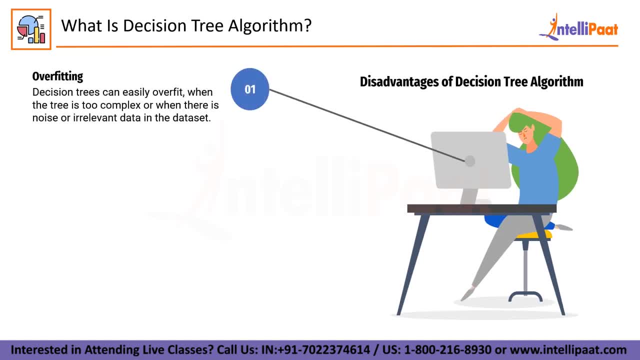 note that this algorithm can easily over fit the training data, especially when the tree is too complex or when there is noise or irrelevant data in the data set. This can lead to poor generalization performance. on new data, I mean, this algorithm might not make right predictions. 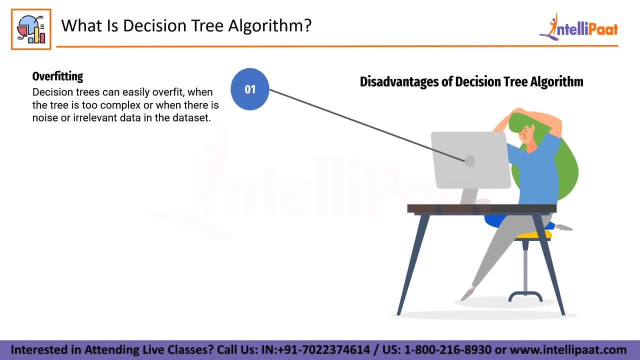 if it is trained over the noisy data. Second disadvantage appears in terms of bias. Decision trees can be biased towards features that appear earlier in the data set. For example, this algorithm can be biased towards features that appear earlier in the tree or have more. 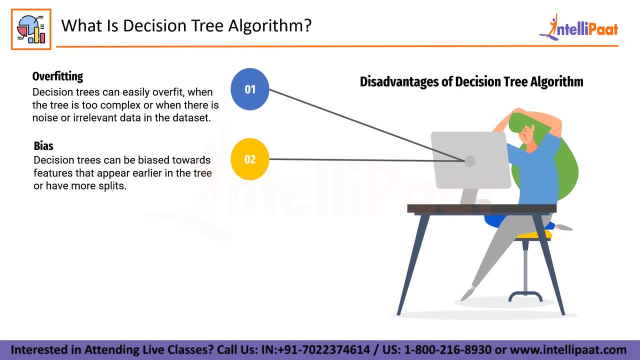 splits, leading to sub-optimal performance. Next downfall of this algorithm is that it can become quite unstable with little variations. Even the small variation in data can lead to different tree structures, which in turn, can make things difficult for interpreting the results or even for comparing models. Another thing I want to make clear is that 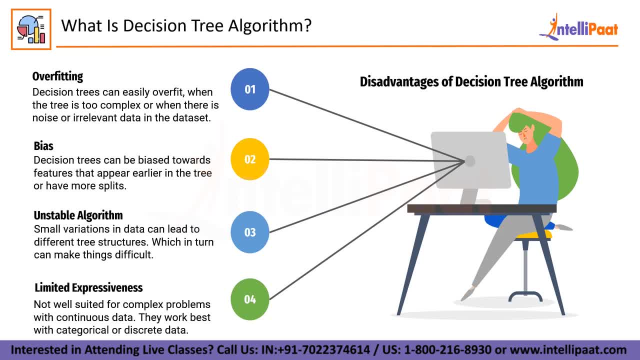 this algorithm is not meant for huge data sets. With a multitude of important features, it has very limited expressiveness. Decision trees are not at all well suited for complex problems or problems with continuous data, as they have limited expressiveness. They work best with categorical or discrete data. 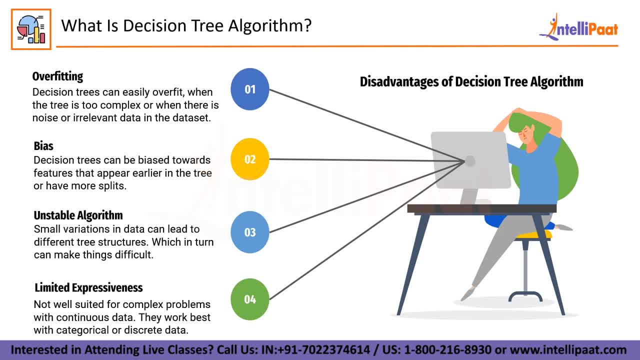 and are less effective for problems that require more sophisticated modeling approach. Alright, the reason behind telling these disadvantages is that I want you guys to note that this algorithm is not really best suited for complex data sets, But by putting it to use and doing little, 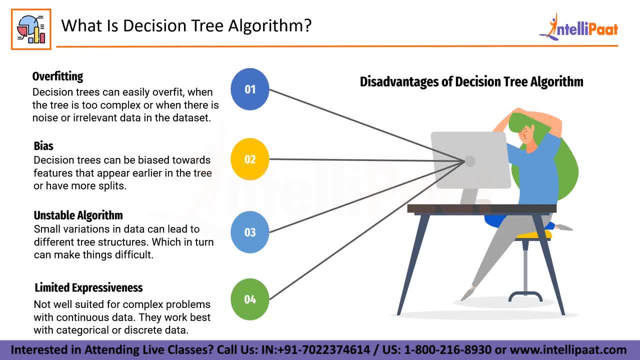 changes here and there, all of these disadvantages can be removed successfully. We'll discover all those advanced algorithms named as random forest pruning, XGBoost, gradient boosting trees, etc. down the line, But for now let's just focus on this basic notion of decision. 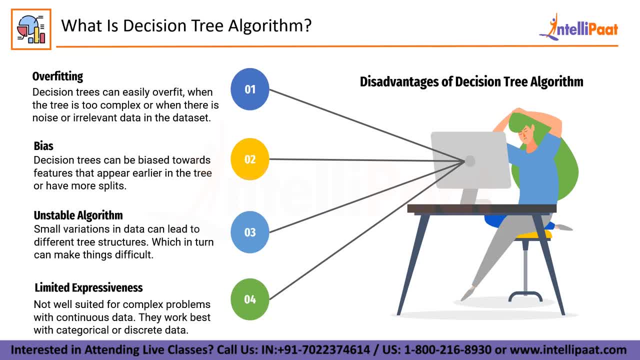 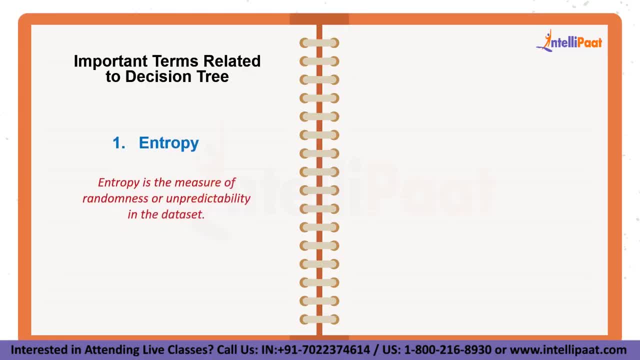 tree algorithm. Next thing we shall look into is about the important terms related to decision trees. We'll start with a term called as entropy. In simple terms, entropy is the measurement of randomness or unpredictability in a data set. I mean the more the classes in the data. 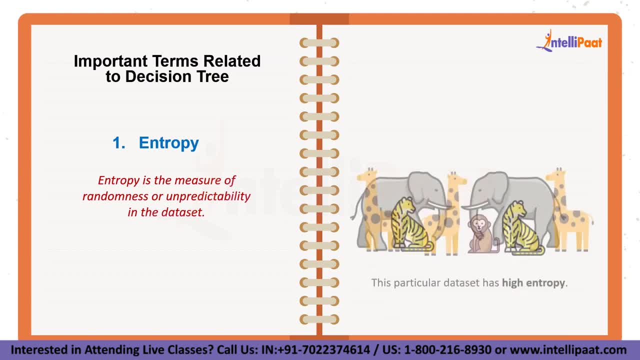 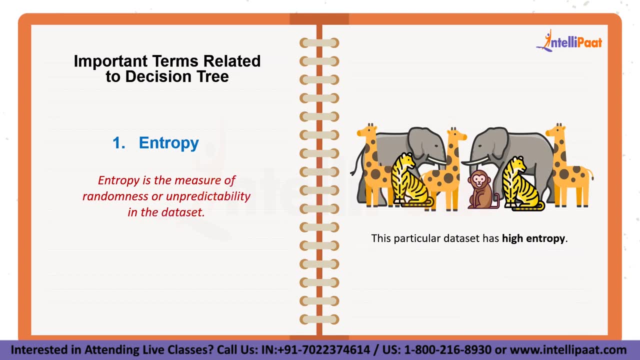 set more the entropy it will have. This image over here represents the sample with high entropy. You can see different types of animals clubbed and mixed together in this image. Also, you'll have to consider the features of each and individual animal to select the 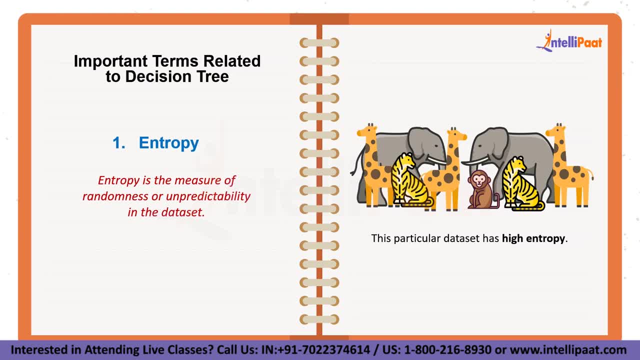 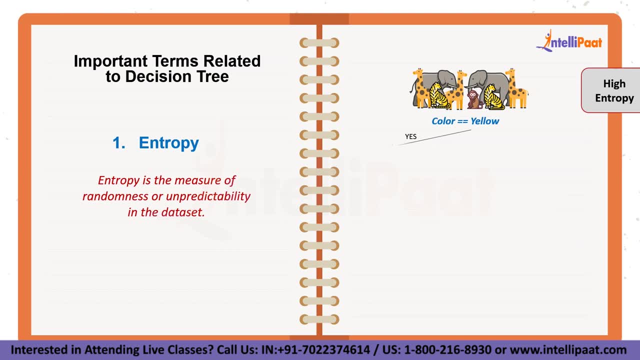 animal and segregate them into their categories. So we can say that there is definitely some unpredictability and randomness in this sample. But now let's say we use the logic of decision trees. First we'll check for the color of animals. If the color is yellow, then animal. 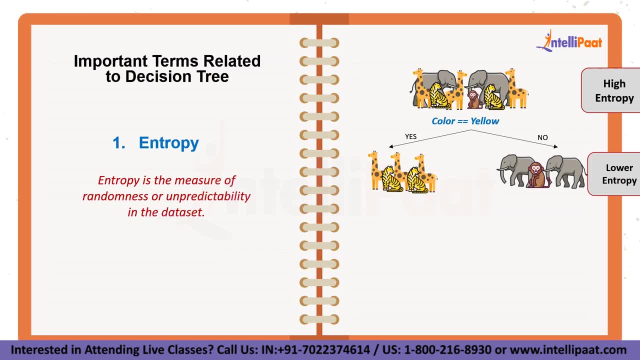 will arrive at the left hand side, otherwise they'll go to the right hand side. Here we only have 2-2 different types of animals, So definitely the entropy at this stage is much lesser compared to the previous state. Now we check for neck length. If the neck length is more than 5, then the animal move. 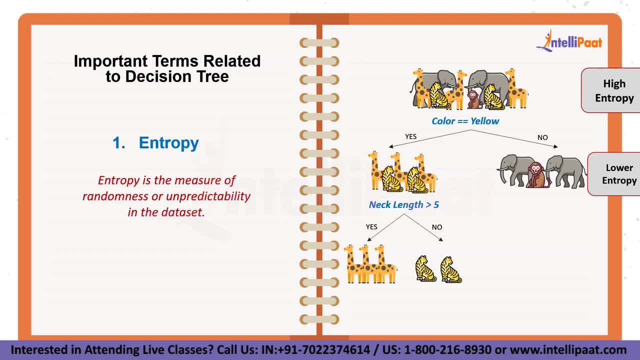 to the left side and other animal will go to the right side. Similarly, we'll check other group for length. If length is more than 10 feet, animal is going to be elephant, otherwise it is going to be 0.. Now, at these leaf nodes we have got the distinct classes. 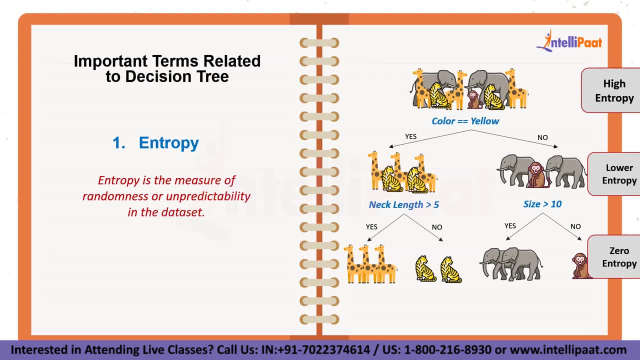 and there is no randomness at all. So definitely the entropy for these leaf nodes will remain 0.. We can say that entropy is a kind of learning strategy that helps in making decisions. The goal with this strategy is to reduce entropy such that the overall entropy reaches the 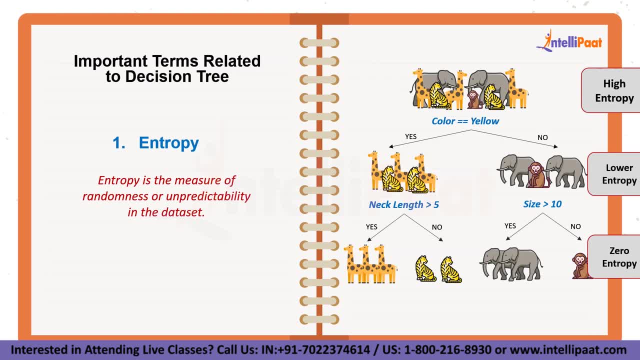 least possible value with the help of optimal decision making. The formula to calculate entropy is h. i is equal to negative summation of p i k log to p i k. Now here the base for log is going to be 2 and p i k is the probability of the. 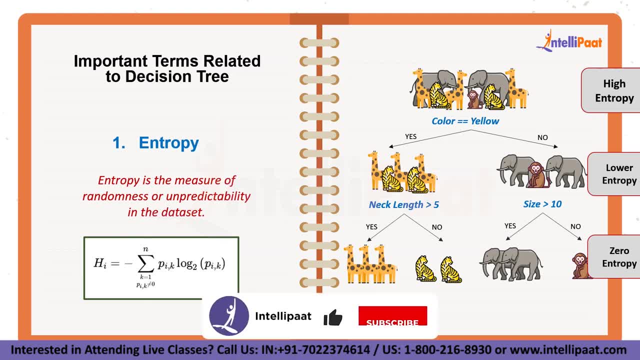 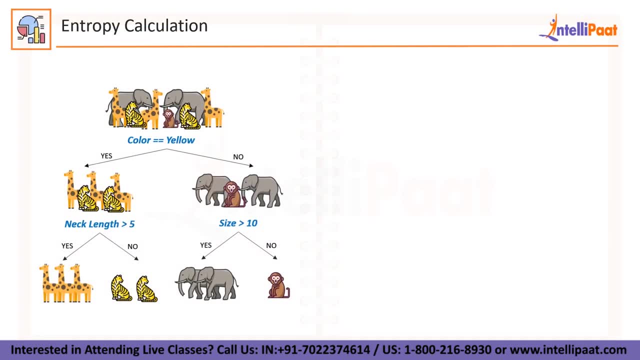 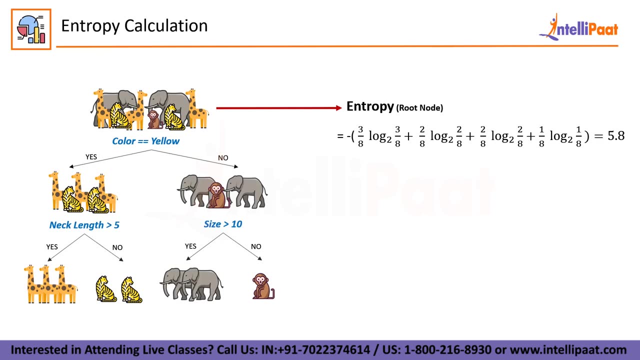 positive and negative class i at the particular node. Let me show you how this work in real time. So, basically, what we have to do is calculate the entropy for each stage for this given sample over here. So the entropy at root node or beginning stage will be something. 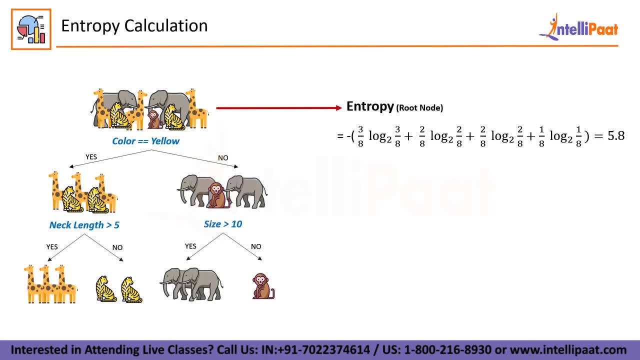 like this. So in this sample at root node we have 3 different giraffes, 2 tigers, 2 elephants and 1 monkey. So overall we have 8 animals- Our sample at root node will be- out of which 3 are giraffes, So 3 by 8, log base, 2, 3 by 8 plus. then we have 2 tigers. 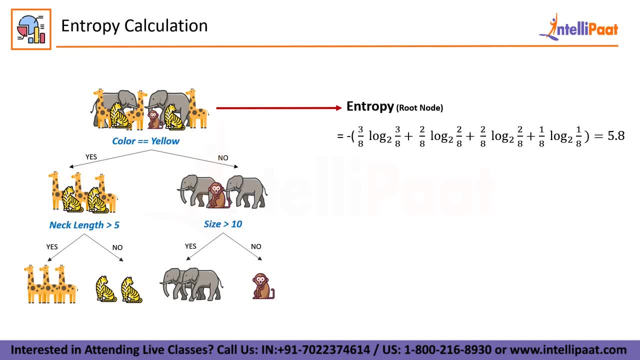 So 2 by 8, log base 2, 2 by 8 plus. then we have 2 elephants, So 2 by 8, log base 2, 2 by 8 plus. then we have 1 monkey, So 1 by 8, log base 2, 1 by 8.. Now, if you calculate this: 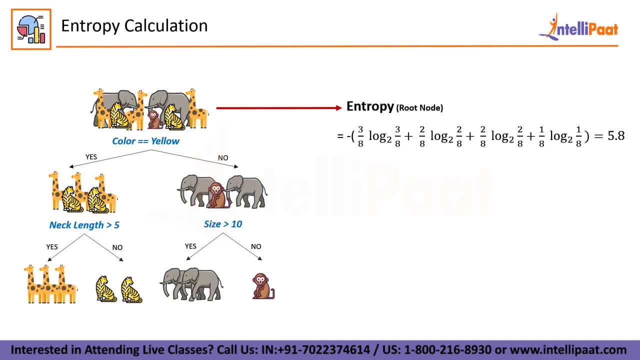 the output that you will get is 5.8.. Now here the entropy that we are getting is quite substantial. Generally, in an ideal machine learning setup, the entropy is measured between 0 and 1. It should not go above 1.. But all of it is quite data dependent, Depending upon. 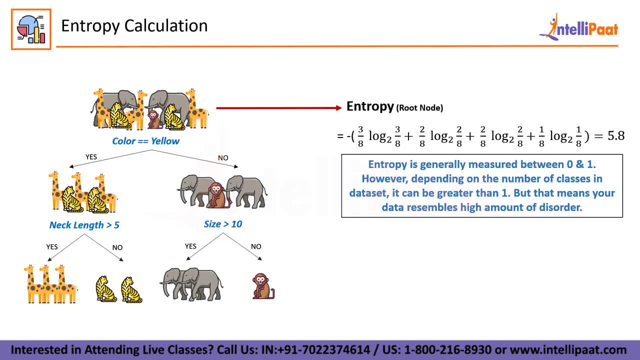 the number of classes in the dataset, it can be greater than 1.. What that simply means is your data has a very high level of disorder And this algorithm is not at all good fit to get the classification job done. But for just example sake, let's see how we can get the classification job done. Let's 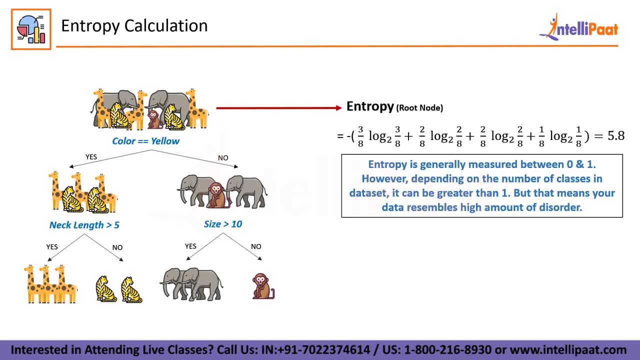 start with the second term. For the samples sake, we are considering this calculation over here as a valid one. Now moving ahead. for this rightmost node at second level, the entropy will be around 0.91.. whereas it will be 0 for all the samples at leaf node, The. 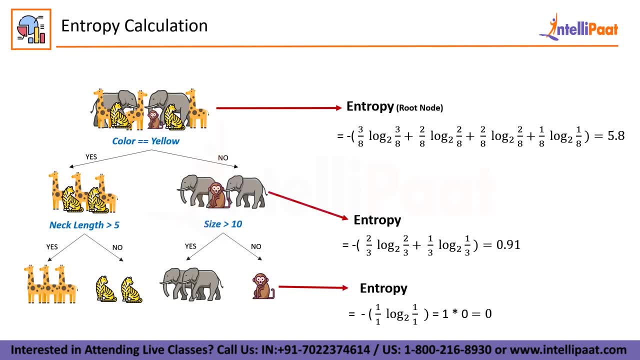 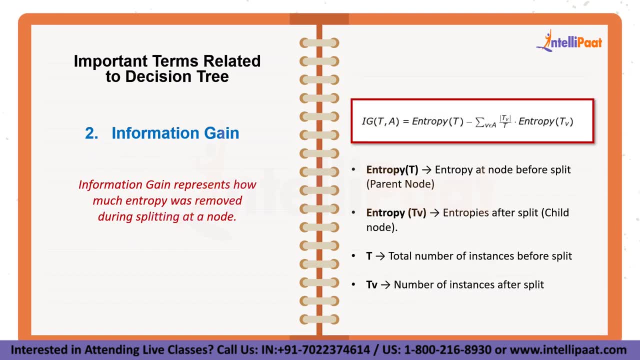 computation for them is given on the screen as well. Now the next term we have is information gain. It represents how much entropy was removed during splitting at a node. Higher the information gain, more entropy was removed. Therefore, it is lighter than 0 at leaf node Also, even more entropy was removed at leaf node, So 0 for all the samples at the node. Now the next term we have is information gain. It represents how much entropy was removed during splitting at a node. Higher the information gain, more entropy will be removed. So if we do this step, 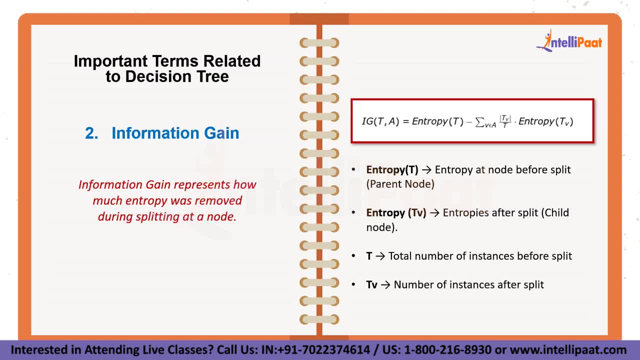 Entropy is removed. Hence during training the decision tree best splitting is chosen which have maximum information gain. Now the formula to get information gain is entropy T minus summation of Tv divided by T into entropy of Tv. Here entropy of T is entropy at node before split, ie parent node. Entropy of Tv represent entropies after the. 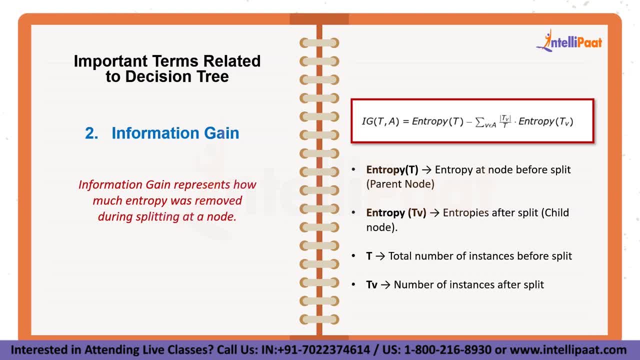 split, ie child node T represents total number of instances before split and Tv represent number of instances after split is done. Basically, you can consider information gain as a difference between Entropy at the parent node and Entropy at the child node. All right now, this is pretty easy to understand. The next strategy that we have on our list: 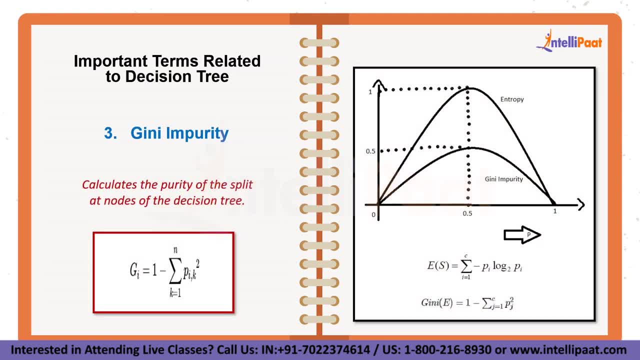 is Jinnah impurity, Jinnah impurity, the purity of the split at nodes of decision tree. The mathematical equation of Gini attribute at ith node is given by Gi, is equal to 1 minus sigma Pik. square Pik is the ratio of class. 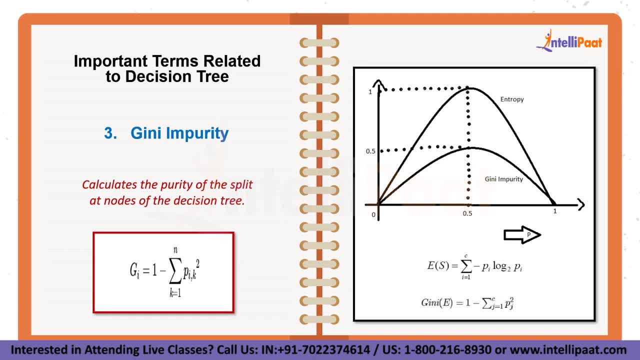 k instances among the training instances in the ith node, Unlike entropy, the value of Gini impurity varies between 0 to 0.5.. A node is pure when Gini attribute is equal to 0, that is, all instances are of a same class. Now let me show you guys the computation. 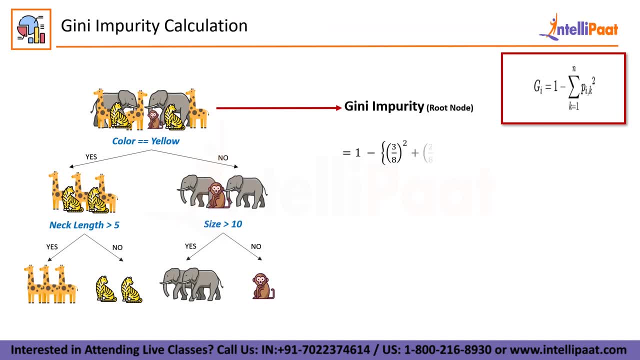 for Gini impurity, for our previous example itself. Now, here, at the root node, the Gini can be calculated by 1 minus sigma Pi square. Alright, So we'll have to consider the probability of getting giraffe, probability of getting tigers, probability of getting monkey, and 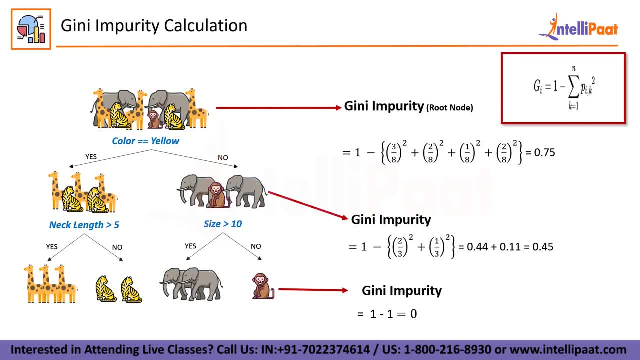 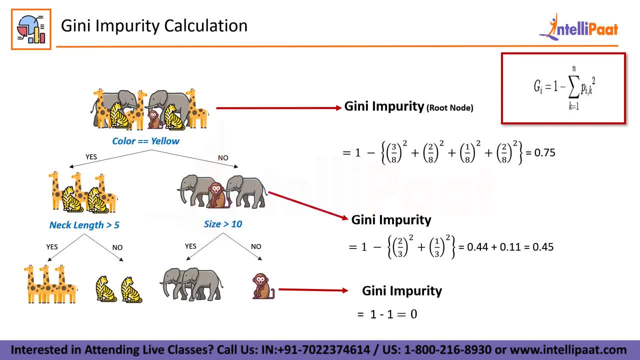 plus 2 by 8 square, plus 1 by 8 square, plus 2 by 8 square, which equals to 0.75.. Right, Which is again exaggerating the range that we have been talked about previously, And 0.75 is quite substantial than 0.5.. Now the reason behind we are getting this kind of. 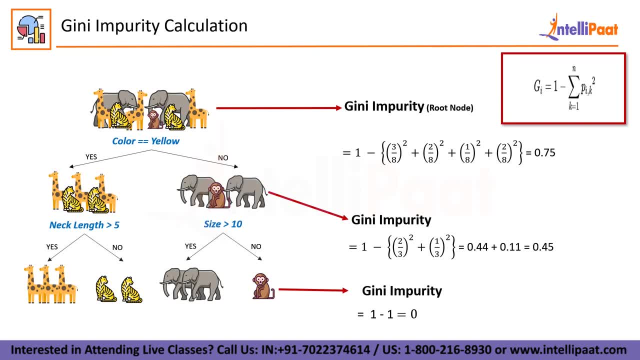 number is that we are just considering few features and samples, whereas number of classes is quite substantial. Basically, the data we have has a high degree of randomness. So just for understanding sake, let's say this is a valid example. Now let us consider the Gini impurity values for 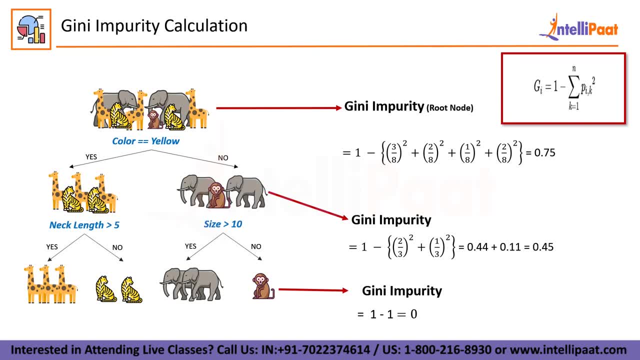 few more samples. Now for this particular right node, where we have two elephants and one monkey, the Gini impurity will be 1 minus 2 by 3 square, that is the possibility of getting elephants, plus 1 by 3 square, that is the possibility of getting monkey. So the value we are getting. 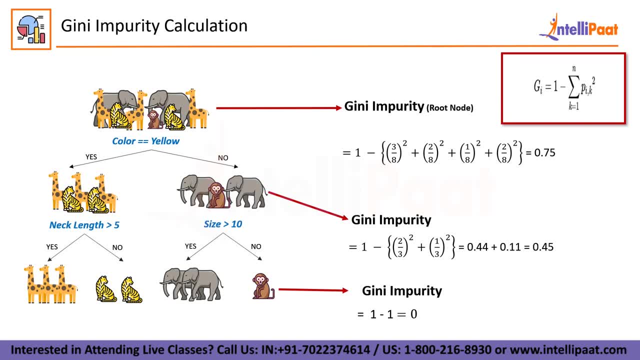 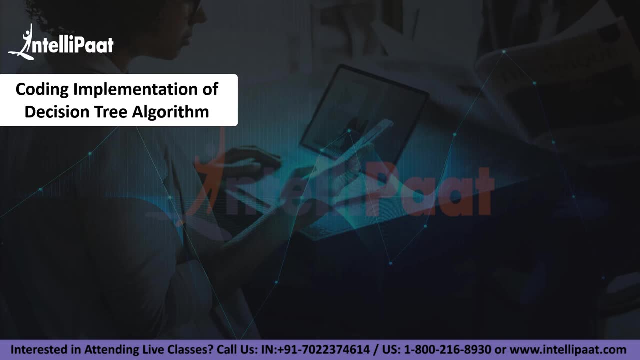 over is 0.45 and at the leaf nodes we are getting 0.. Alright, that's almost everything you need to know before implementing a decision tree algorithm. I hope this information is clear to all of you guys. Let's move ahead and develop. 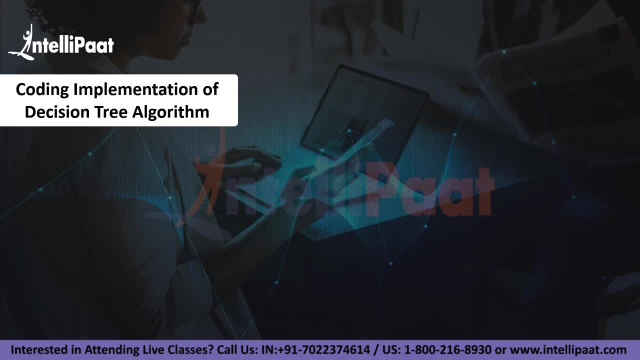 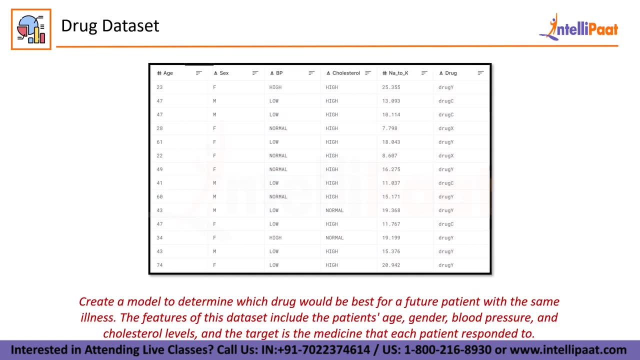 a working decision tree classifier model. For this purpose, we will be using a medical reports dataset that we have over here. This dataset basically entails which drugs work on patient given certain parametric reports. Now for clarity, let us imagine that you are a medical researcher compiling data for a study. You have collected data about a set. 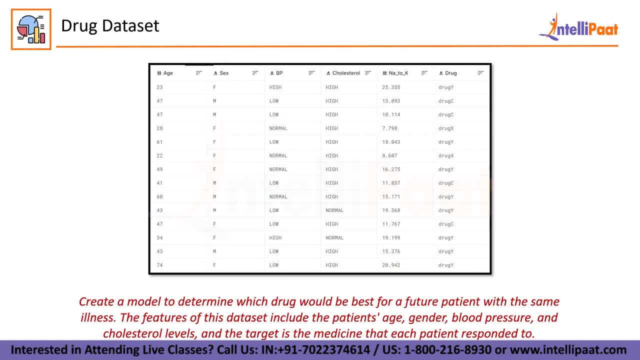 of patients, all of whom suffer from the same illness. During their course of treatment, each patient responded to one of five medications: Drug A, Drug B, Drug C, Drug X and Drug Y. Now the part of your job over here is to build a model to find out which drugs work. 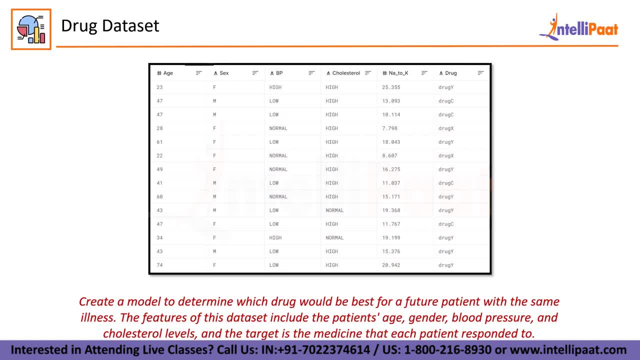 and which drugs might be appropriate for a future patient with the same illness. The features of this dataset are age, sex, blood pressure and the cholesterol of the patient, And the target is the drug that each patient responded to. Alright, now I hope you guys understand that this is basically a multi-class classification. 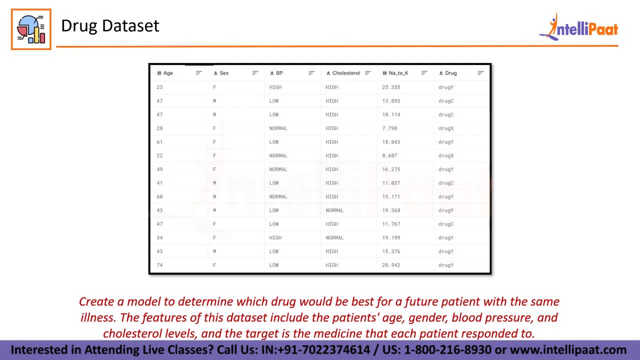 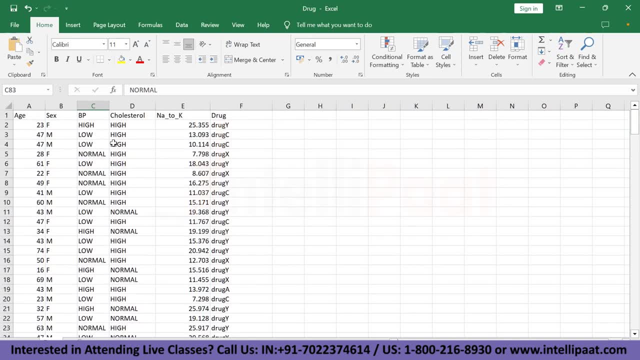 problem, and we are going to solve this using the decision tree classification approach. Now let's move ahead and develop a working decision tree classifier model. For this purpose, we are going to use the Excel file of our dataset that contains different features, such as age. 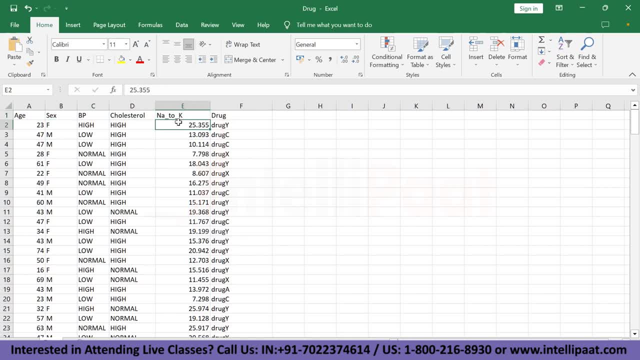 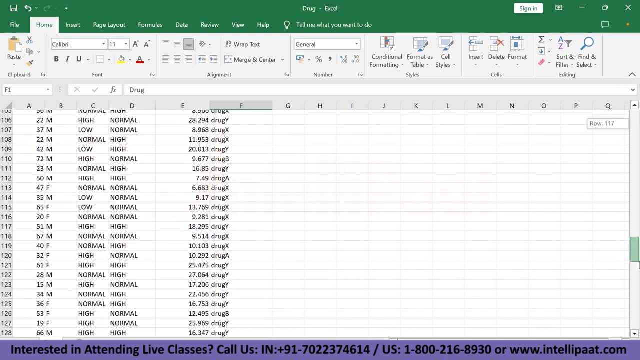 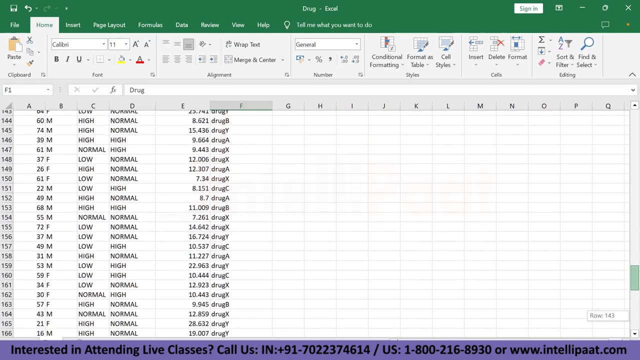 sex, blood pressure, cholesterol, sodium to potassium ratio and the name of drug, which is again a label. So we have around 200 records over here. So let us import this data to our Collab notebook and get us started. To begin with, we'll upload the drug data to our Collab notebook, So 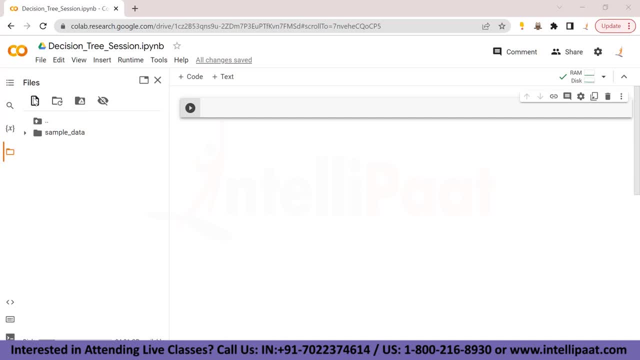 I'll go here, go into the upload section and I'll load this drug data over here. Alright, so we have successfully uploaded the drug data on Collab environment. So all we got to do is import this data into our Collab notebook, and for that purpose we are going to require the pandas library. So 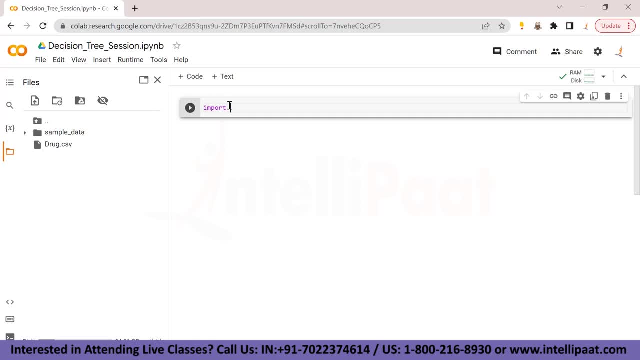 first of all, let me import this library framework, And then I'll store my data inside data frame named as df using the function pdread underscore csv, And inside it I'll pass the name of my data file, that is, drugcsv. Now let us check if our data 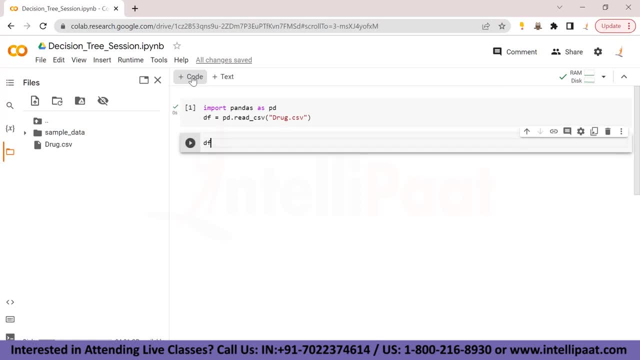 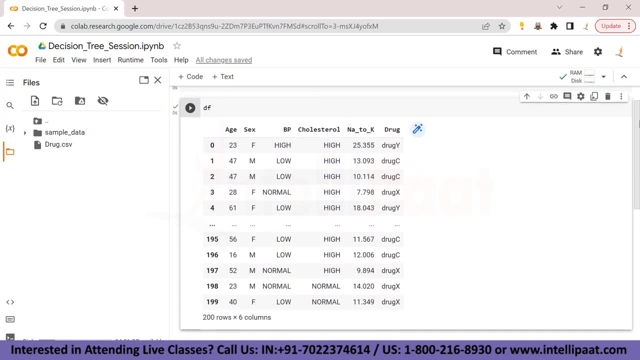 has been saved inside this data frame or not. For that purpose, we'll simply type df and run the block, and it shall return our data set. Alright, so here we can see that our data has been successfully loaded into our Collab notebook. 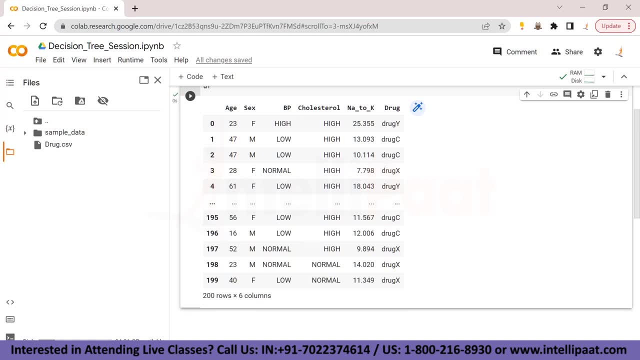 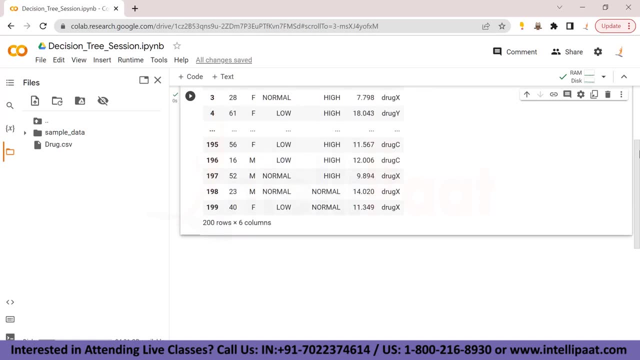 I mean, we can see that there are 200 rows and 6 columns in our data set, which is we already validated in our Excel sheet overview as well. Now, moving forward, we are going to require multiple functionalities, So let us load all of those. 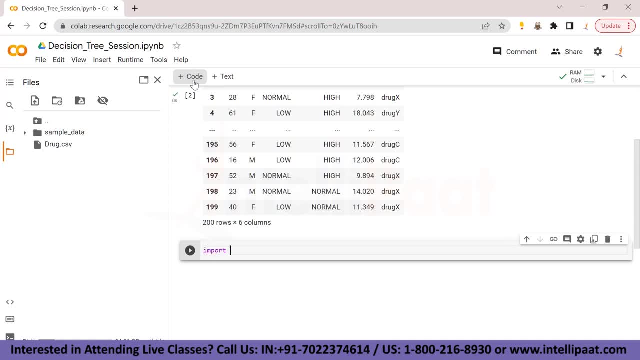 functionalities such as import numpy as np. We are going to require seaborn for visualization purpose as well, So we'll load it here. import seaborn as sns, We'll import matplotlib as well And we'll run this block. Okay, now it's time to move on to the next stage, called as data preprocessing. So with this stage, 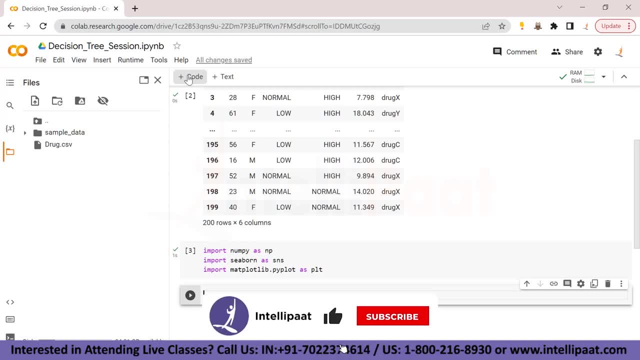 we are supposed to deal with duplicate records, missing values, non-numeric values available in our data set, Because these things can impact learning of our algorithm tremendously. First of all, if data is not provided in meaningful manner, the model won't be able to learn pattern. 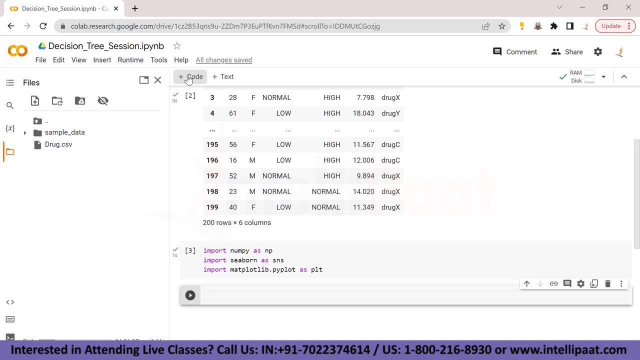 at all. So preprocessing is not a good idea. So let's move on to the next stage, called as data preprocessing. So preprocessing is quite a critical step of machine learning problem solving roadmap. Let us deal with null values for first. The NAND field in data set represents 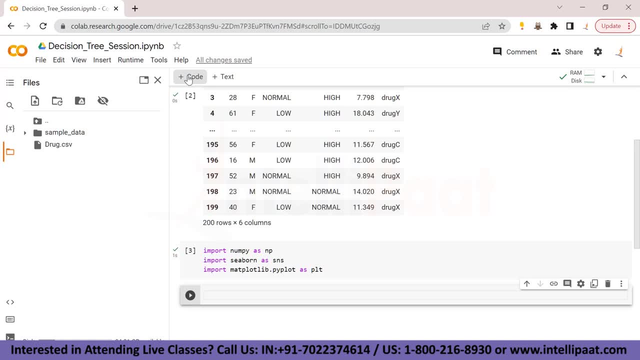 that there is no record of particular feature in that specific row And the function that allows us to check that is isna. This function returns the Boolean mask of our original data frame where it highlights true for the missing value field. However, the 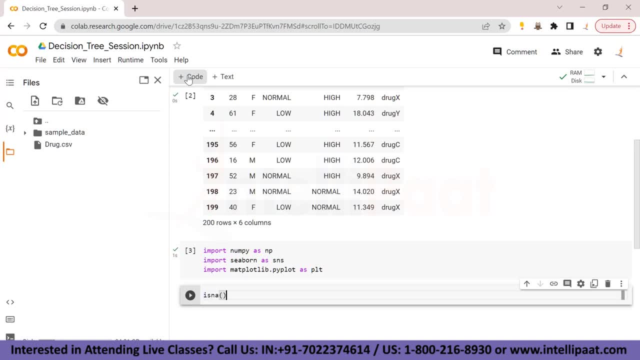 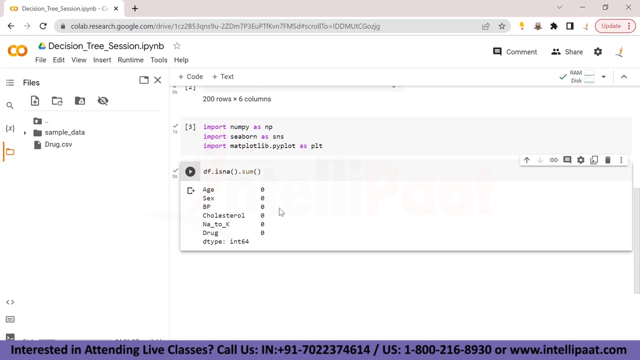 happens when we put isna clubbed together with the sum function. When we do this, we can have a nice list of non-null values, that too, column wise. So if I run this block of code, you'll see that there are no null values available in our dataset, and all of the columns. 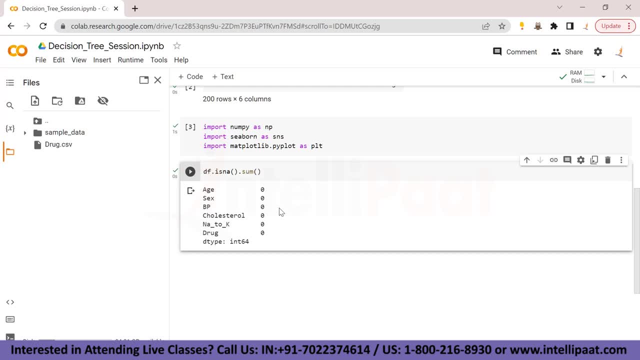 have some sort of values. I mean, there is no null record available in our dataset. The next thing is checking for duplicate records in data, And for that purpose we are going to use duplicated function. So this duplicated function basically returns a Boolean series. 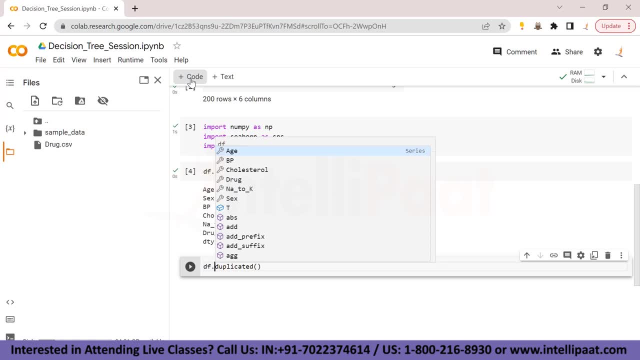 of the same length as of our data frame, where each element is true if the corresponding row in data frame is duplicate of a previous row. Now let me show that over here. So if I pass dfduplicated, you can see that it is creating. 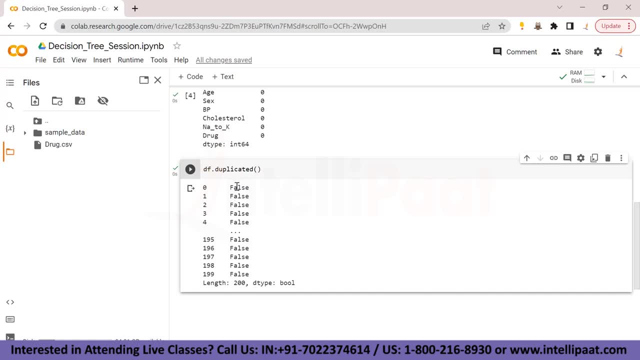 series object where you are getting all the false record. That means there are not really duplicate records available in our dataset. But to make it more understandable, if I put it inside the data frame object, Okay, It will only return the record which is truly duplicated. And here you can see that there. 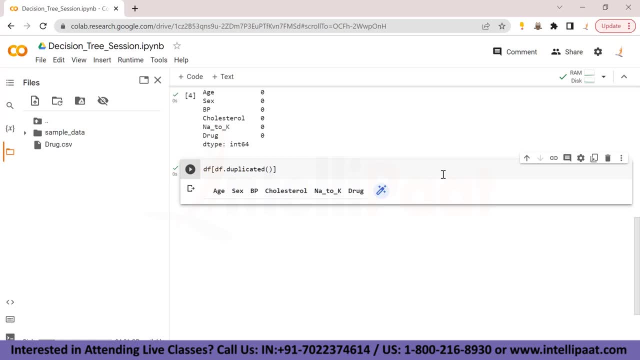 is no record shown on our screen or console. So that means there is no duplicate record present inside our dataset for now. Next, moving forward, Let us visualize the contents of our dataset. So let us first use the dfinfo function to 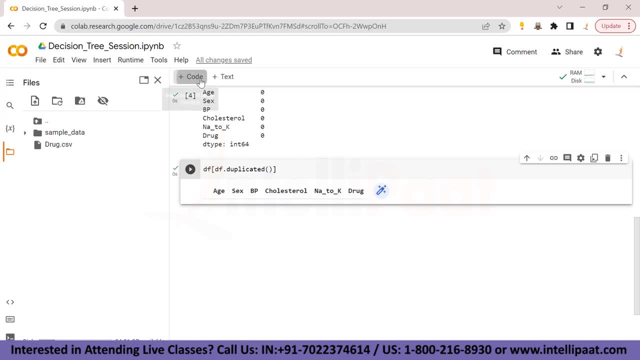 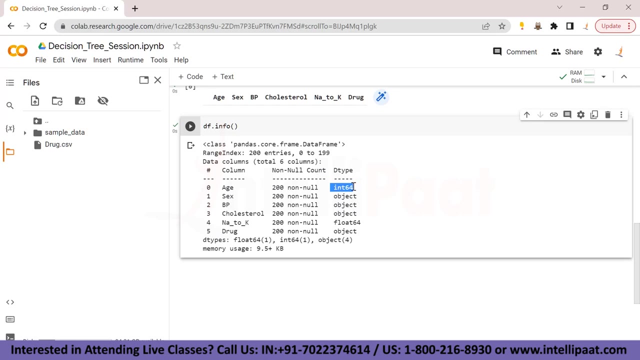 know about different data types of our features. So we will use dfinfo And once I run this block you can see the data types of our columns. So each column has 200 non-null values And the data type for this particular feature is integer. For drug, we have object type. 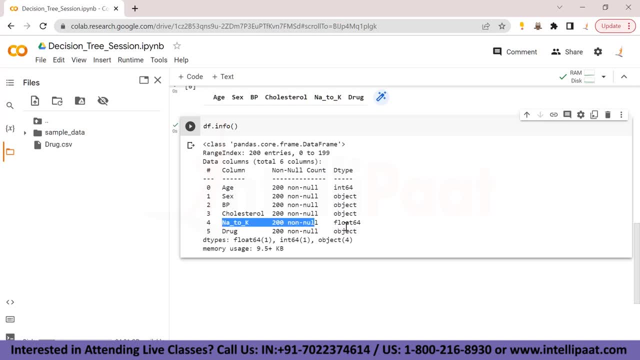 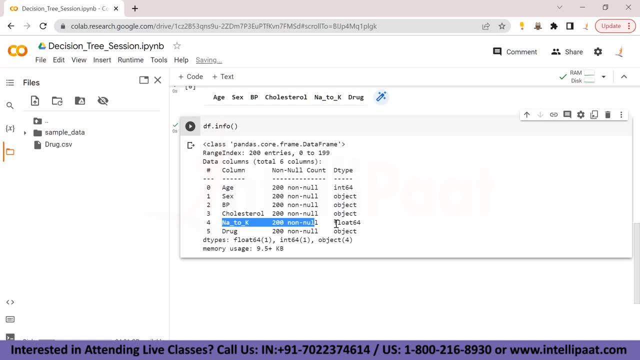 we have the object type. For sodium we have the object type. So basically for whole of our data four features are of object type. that means the categorical type, and then we have one float and one integer type feature as well. Now, for visualization sake, we will look into the sex and drug column graphs. we are 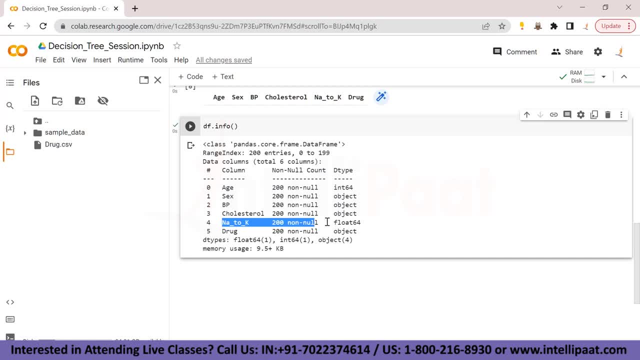 going to use bar plot for that purpose. So first of all let us add a new coding block, And here what will do is will say x is equal to dfsexvalue underscore counts. So basically this will return the tally of different values available inside this sex column. So basically we just 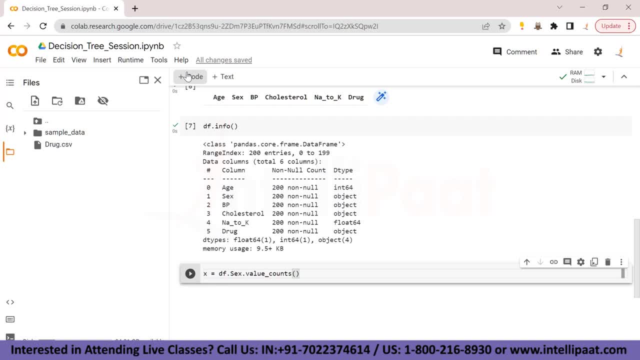 have two values, that is, male and female. So it will represent how many male records are there and how many female records are there, And we want to print that. So we'll use print x over here. After that, we also want to represent this data with the help of countplot. So 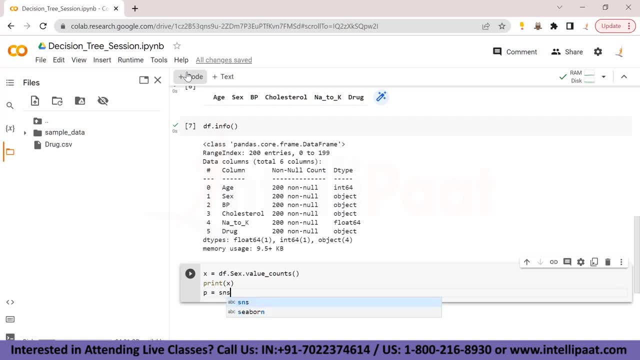 we'll use. p is equal to snscountplot and inside it our data will be equal to df And the titles that we want to give are definitely equal to df. And finally, will be the records of sex, that is, male and female. Alright, And I'll use. 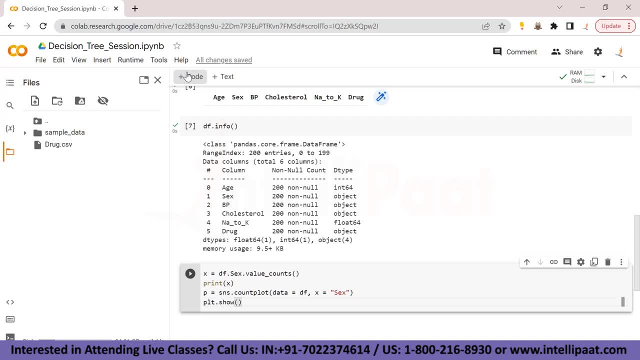 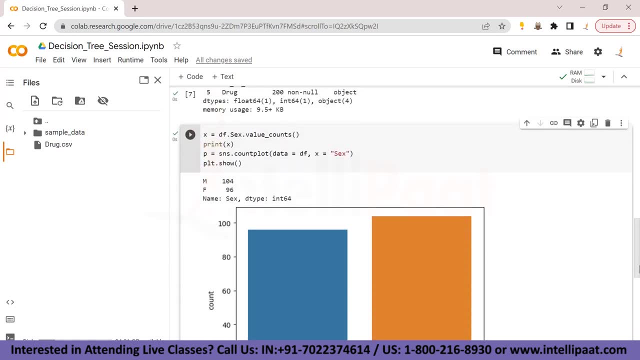 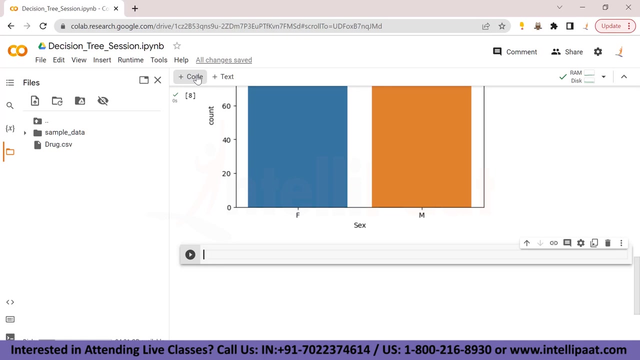 pltshow function to present this graph inside my console. Now, here you can see that we have 104 male records and 96 female records. Now next, we also want to visualize drug column as well. This drug feature is again a categorical feature. So what we can do is we can copy. 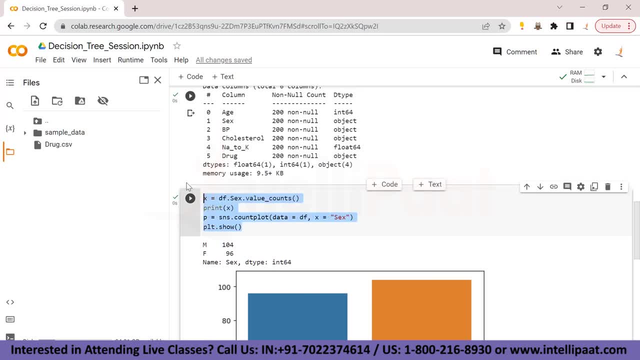 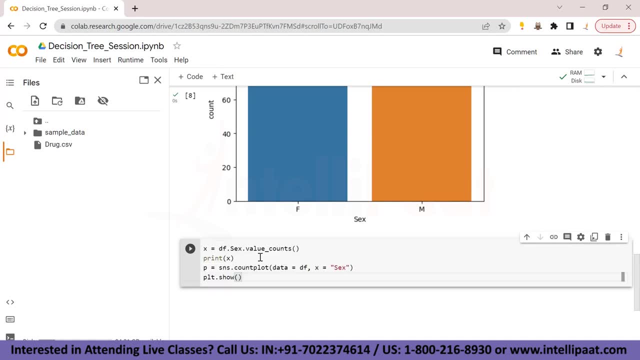 this code above and just change few parameters to get the graph for drug column. So what we'll do is we will set the titles to drug and instead of sex we'll count the different values for drug column. And this shall do it. So once I run this block, we'll see that. 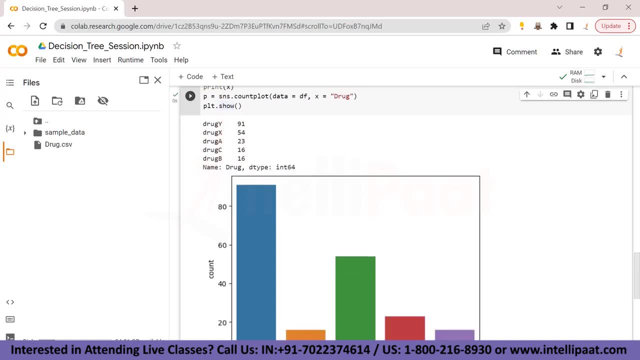 we have 91 records for drug y, 54 for drug x, 23 for drug a, 16 for drug c and 16 for drug b. And here is the graph representing the same statistics. Alright, Now. next we'll be rendering a complex graph over here. With this graph, you can visualize the relationship. 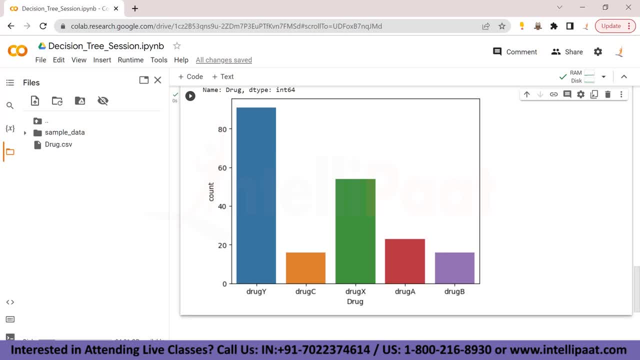 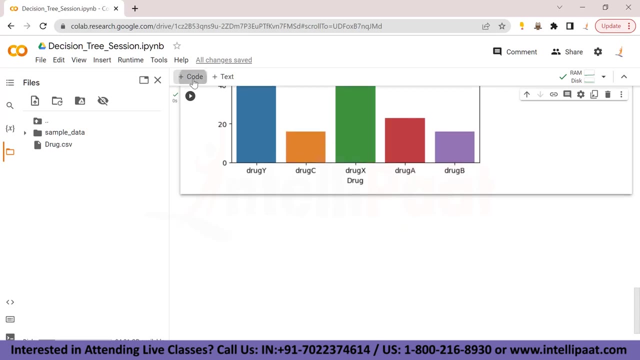 between the feature, age and the drug classes. But in order to create this graph, it is critical that we know all the classes available in out target feature. So what I'll do is I'll print all the unique values of the column drug using the unique function in Python. 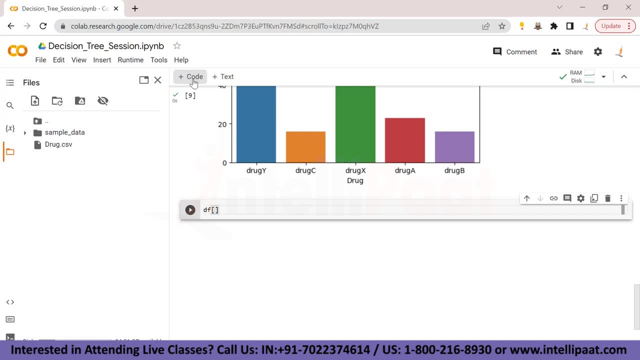 So what I'll do is a df drug return, all the unique values in column. So, like kor run clips for the large term, I'll print all the data as 1f, as Yeah, etc Like that. So there. will be within the self instead of the comma. So using that exclusive now, if you can come into theextero cl in each cl and then whenever you'll be in the external- sorry there will be So as in these be your changes afterwards- You will be in the exp del curr Inside. then select images: Disneyland. 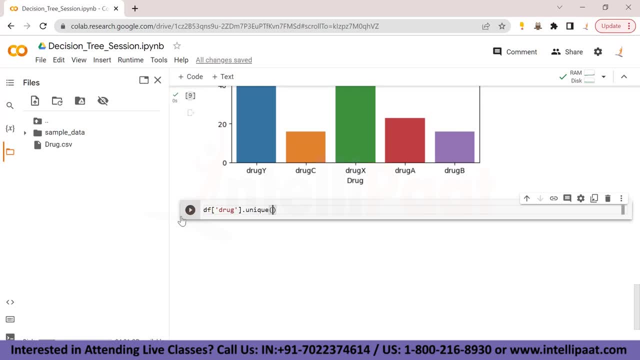 unique values. Okay, this should be capital. Alright. so we have five different records available inside our data frame, such as drug Y, drug C, drug X, drug A and drug B. Now, next, what we shall do is we shall create a figure size to create the graph. So I will. 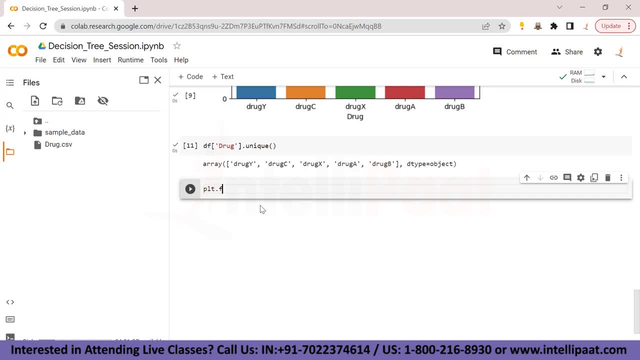 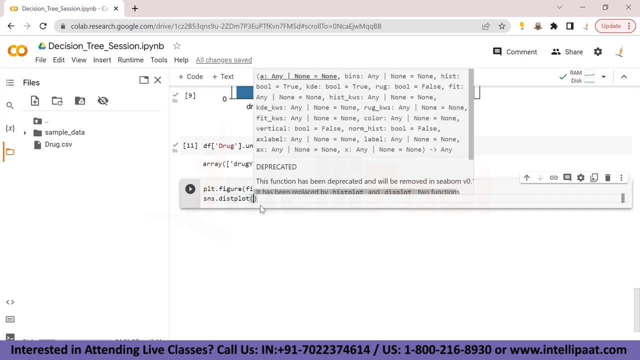 create the plotting area, that is pltfigure, and we will set fixed size to 10 cross 10.. For this visualization, we are going to use the function named as distplot, available in cborn, and inside it we are going to pass nested conditions. So what we will do is we will use df and 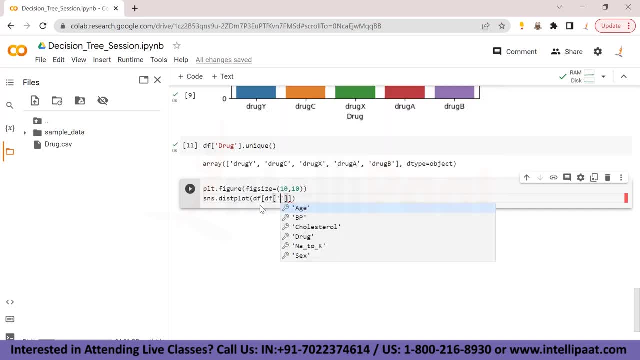 again, df drug. If df drug is equal to equal to Okay, Great drug Y, then we would like to print age records, and the color that we want to set for these samples will be equal to green. now I'll copy this line and I'll paste it five times. 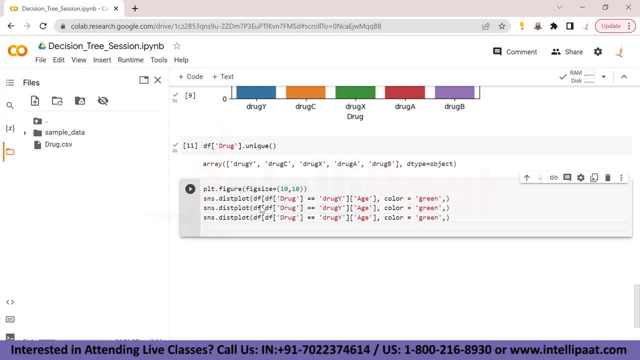 because we have five features or five different categories in our drug column. alright, now I change this to drug X, and the color I'll set for this particular sample will be red, and then drug A, drug B and drug C. for this we'll set color black. 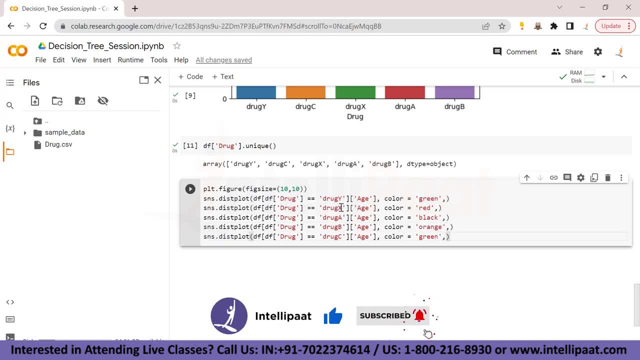 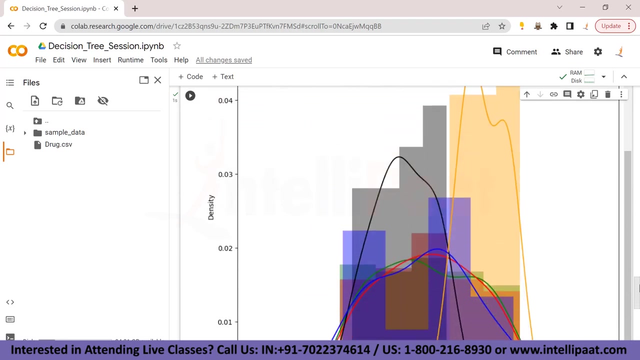 for this we'll set color orange and for this we'll set color blue, and the title that we want to give to this graph is will be age versus drug class, and we'll simply show this graph on our console. now, here you can see this complex visualization. 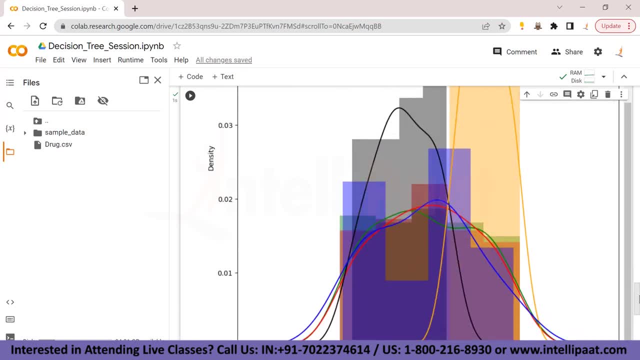 from this particular graph you can comprehend which drug work for which age group and with what probability it worked for them. so basically, from this graph you can understand how the feature named as age is contributing our model to learn towards the label named as drug. alright, I hope this visualization part. 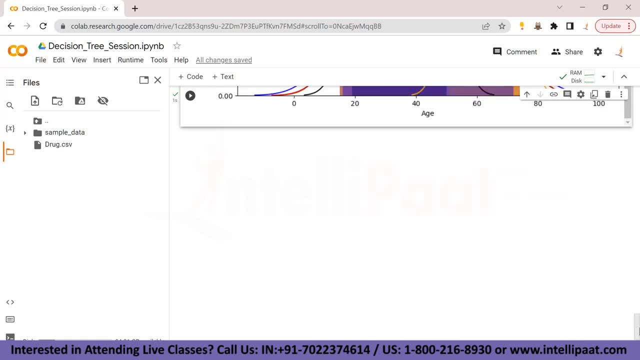 is clear to all of you guys. now let's come back to the undelt part of our preprocessing phase, that is, dealing with non-numeric values. so, as you guys must know, we can use encoding techniques to convert the categorical data samples into the numeric ones. 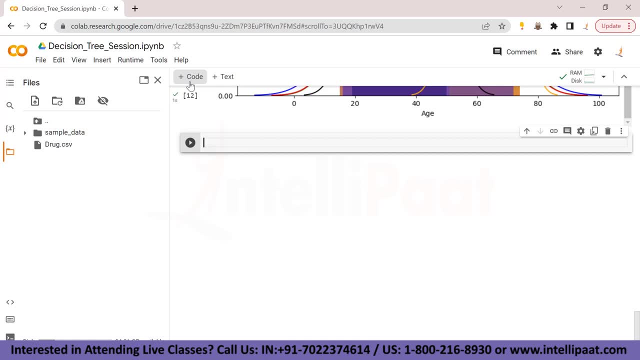 so here we'll use ordinal encoder to achieve this conversion. but before that I'll have to load that ordinal conversion onto our collab notebook. so I'll use the command from sklearncomjp. so I'll use the command from sklearncomjp. so I'll use the command from sklearncomjp. 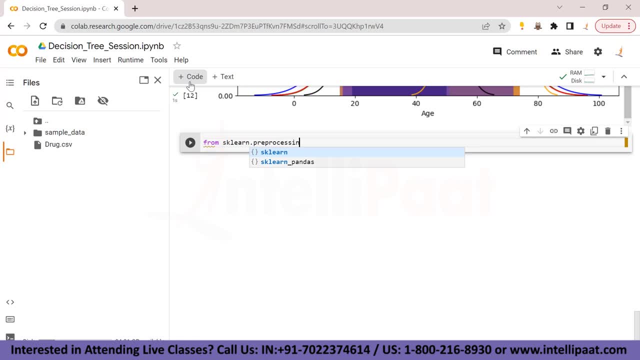 dot preprocessing, import: ordinal encoder. now i'll create the instance of this ordinal encoder. oe is equal to ordinalencoder. So basically, guys, ordinal encoder is a data pre-processing technique in machine learning that is used to encode categorical variables into ordinal variables. It assigns a unique integer value to each category in the variable and transform it. 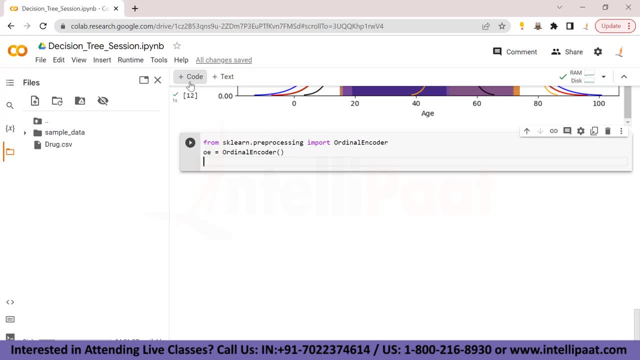 into numerical data. Now we will transform our non-numeric features into numeric ones using this ordinal encoder itself. So what we will do is we will change the records of column known as BP, Blur Pressure, and we will use ordinal encoder and we will use the function named as fit underscore transform. 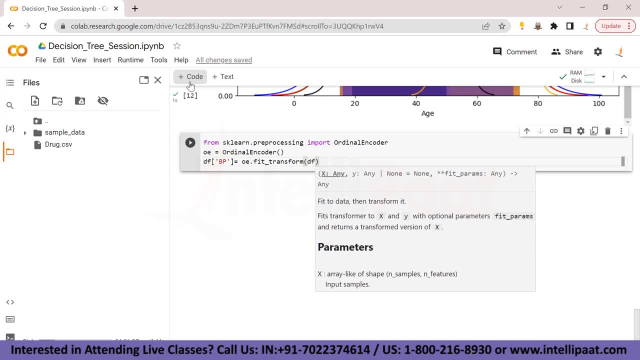 And to this function we will pass 2D object of our BP. So, guys, while passing column as an argument, we are making sure that we provide input in two-dimensional format, because ordinal encoder will return error if you provide series type of object. So just make sure you provide your data frame column inside dual boxes which will convert. 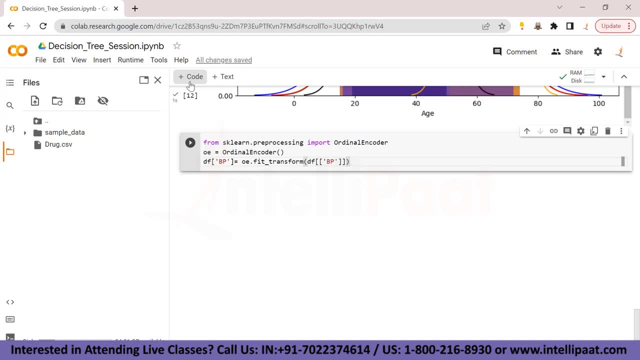 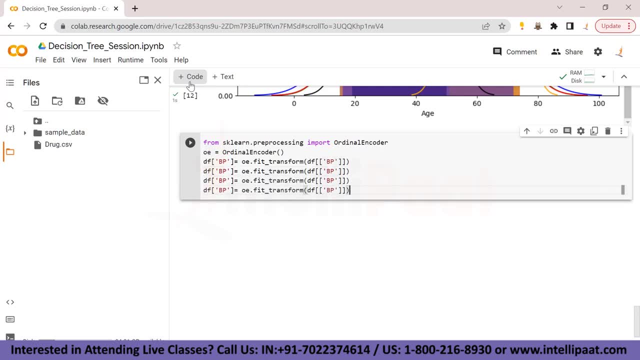 And we will just change the parameters. Alright. So next we will transform the column named as sex, which contain male or female record, And here we will have to pass sex again. Similarly, here we will do cholesterol. Okay, Okay, Okay. 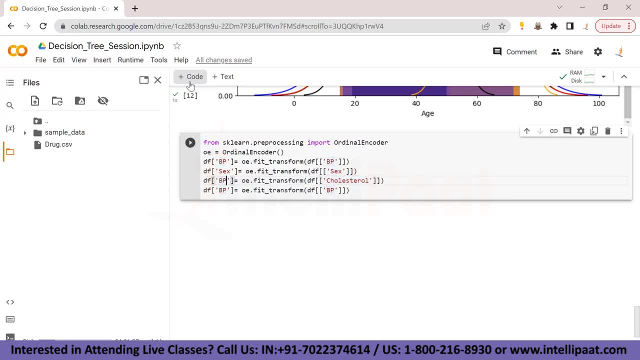 So we will just save this and next we will just write, And next we will transform our label column that is drug, And next we will transform our label column that is drug. Now let me run this block of code. Okay, So let us visualize if this transformation has had happened in our data frame, in our 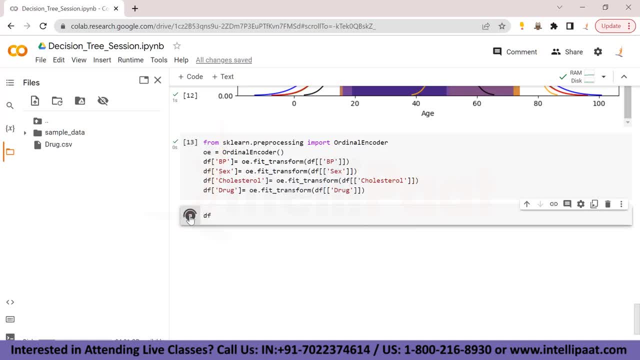 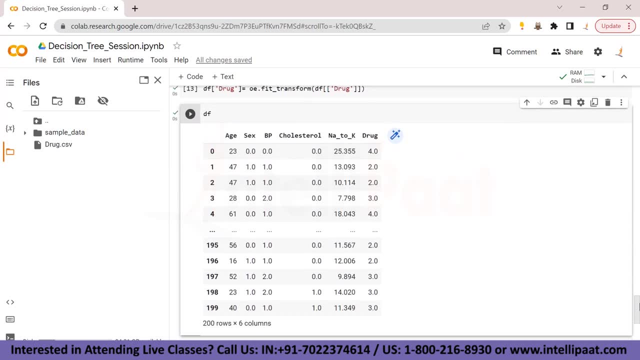 not. we'll just print our data frame, And here you can see that all the categorical records has been converted into numerical ones. Alright, with this step, the pre-processing stage is over. Now we'll perform the splitting of our data set into input and output format, using. 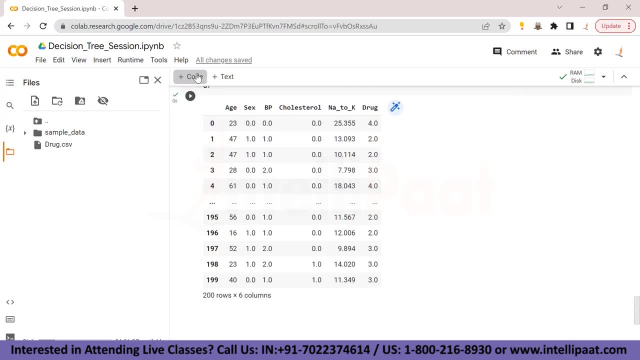 ilog indexing. Alright. so let us get the new block of code and here we'll create input and output format. so x and y- Alright. so x will basically contain all the features of our data set and y will basically contain the label parameter. So first let us put the 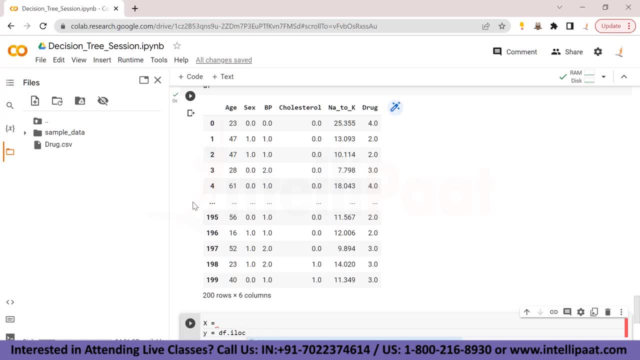 label over here, dfilog, And we'll provide the last column and iscrub it and we'll print it. For data part we will provide all other features except the label feature and for that purpose we will use indexing from 0 to minus 1.. 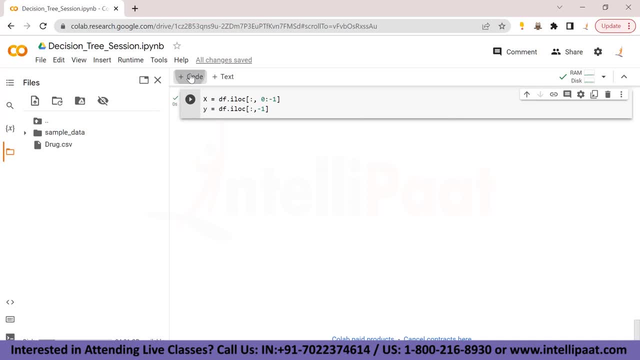 Now let me run this block of code, and here you can visualize the x and y as well. Alright, so there is no presence of label column over here, and let's print y to see the label. Okay, so we have successfully converted our data into input and output format. 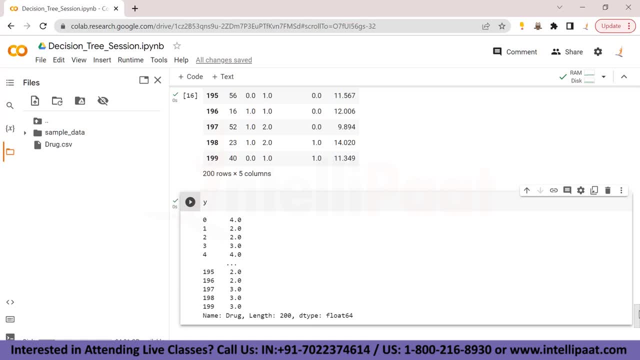 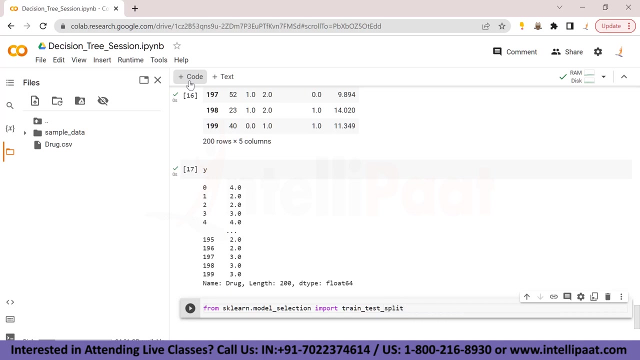 Now we'll import the train test split function and we'll simply break our data into training and testing samples And for this purpose we'll import the train test split function from sklearn dot model underscore selection: import: train underscore- test underscore split. Okay, And now the training split x- train comma. testing split x- test comma: y- underscore train comma. 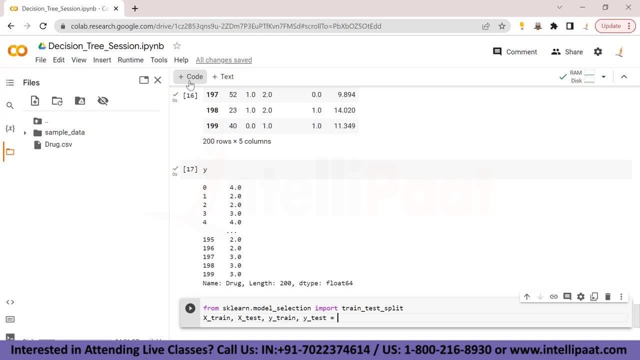 y underscore test will be train, underscore test, underscore split. Here we'll pass the test. Okay, And now we will run the test, Okay, Okay. So here we'll run the test and we'll set the input, then output, then the random state. 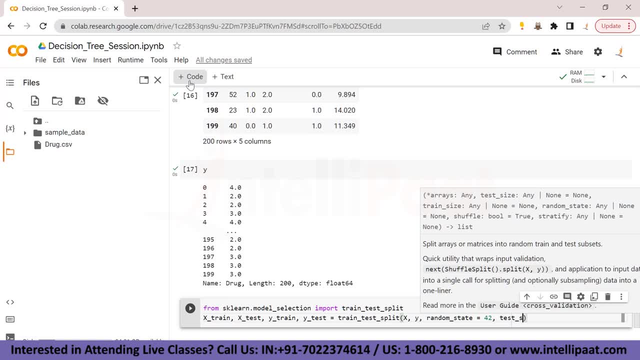 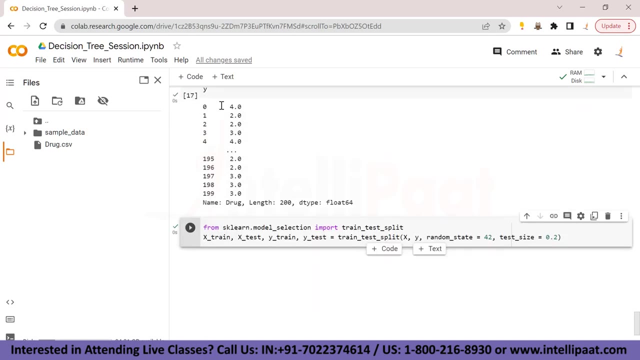 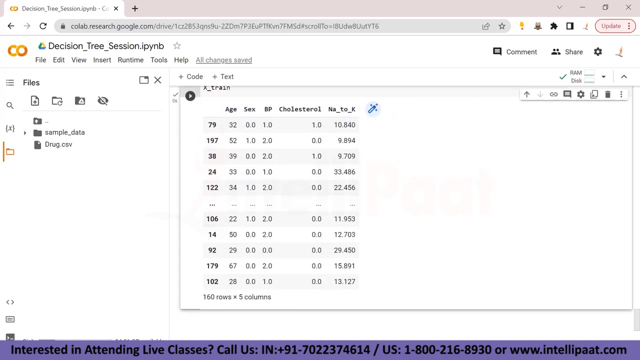 and we'll set test size as 20% of our data, So 0.2.. Now let me run this block of code Here we'll run it, Okay, And now we will import data. Okay, Let us visualize the X train. Here you can see that we don't have label in. 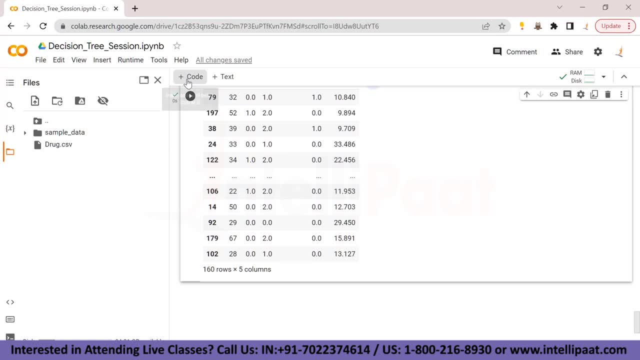 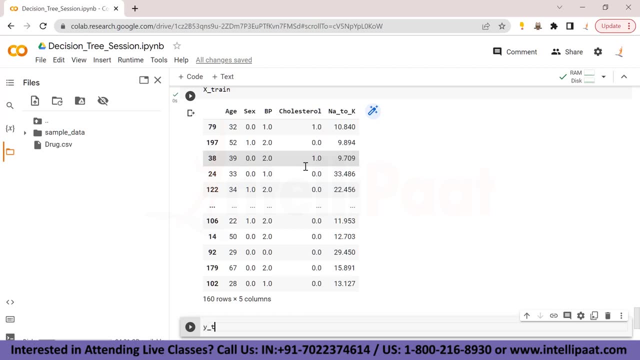 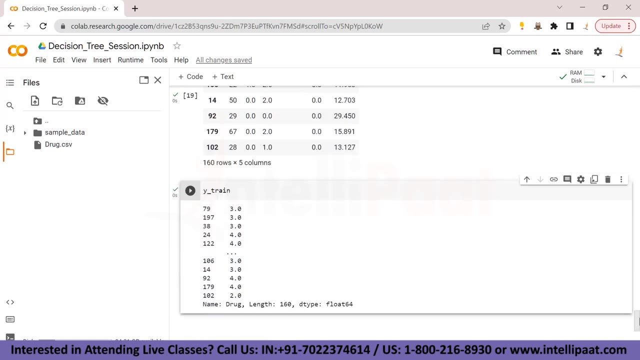 this sample and if we check for X test, we will just found the label, and if we check for Y train, we will get our label Alright. so we have successfully done the splitting of our data set into input output, as well as training and testing samples. Now we have 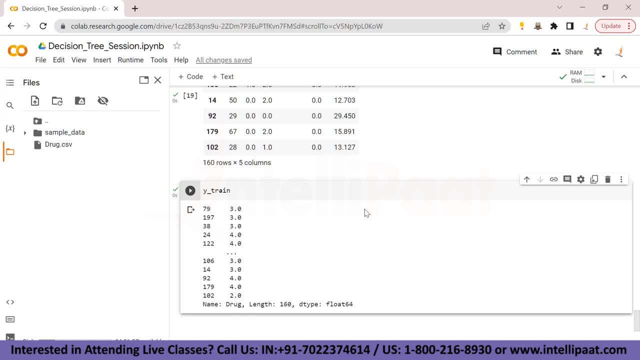 converted our data into something that can be fed to the machine learning model. So, without wasting any time, let's import the decision tree classifier and get to the business of making prediction. For that purpose, I will have to import the decision tree classifier for first. So from sklearntree, import decision tree classifier. 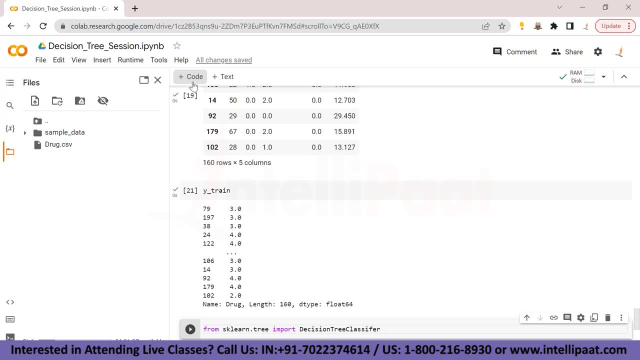 First of all, what we will do is we will use Gini impurity criteria. So let us name the classifier object that we are going to create in next line as classifier Gini And we will create the instance of decision tree classifier And inside it we will set our criteria as Gini. 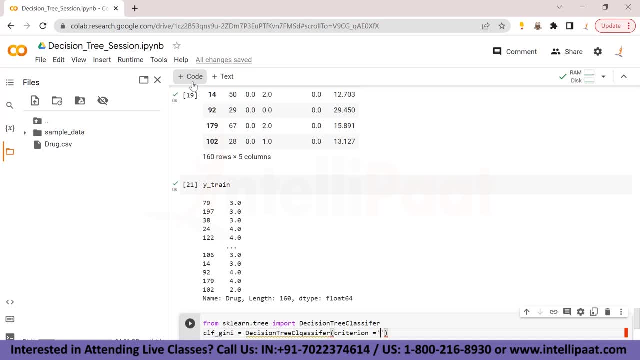 Okay, there is one spelling mistake over here. decision tree classifier. Okay, we will set criteria as Gini And we will set criteria as Gini And we will set criteria as Gini. We will set the classifier object with 분�. We will factor that somewhere inside. 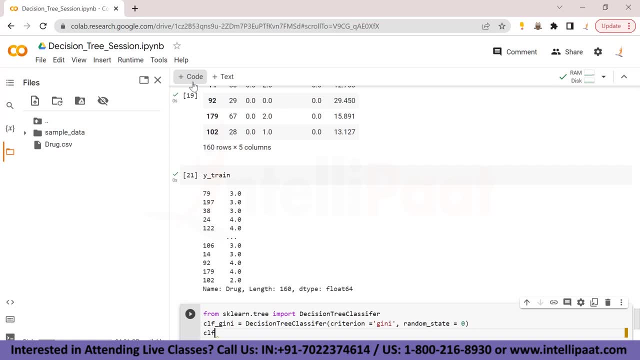 So let us find our specific classifier, Vinenya Gini test. okay, find exactly where the classifier is. define what is the method which we are going to create our instance or a set foreigner whom we are going to be Garcia from this command. our model will pick up the pattern from our available training dataset. 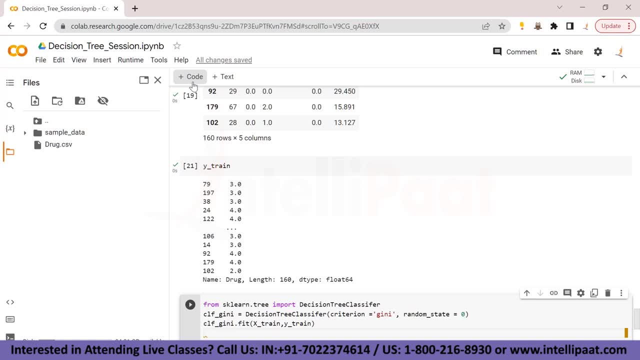 and next what we will do is we will make the prediction and we will store those prediction inside y underscore, pred underscore, gini- named variable and we will use clf, dot, clf, underscore, gini, dot, predict function and inside it will pass a testing sample that is x underscore. 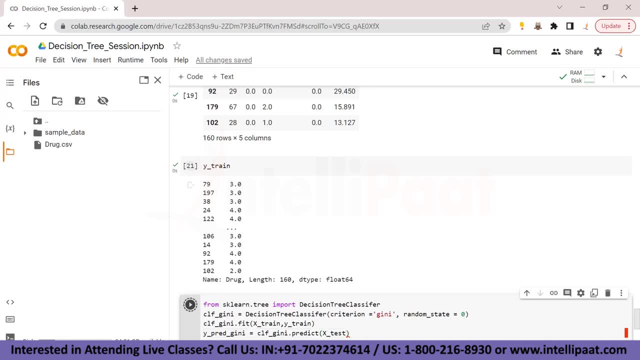 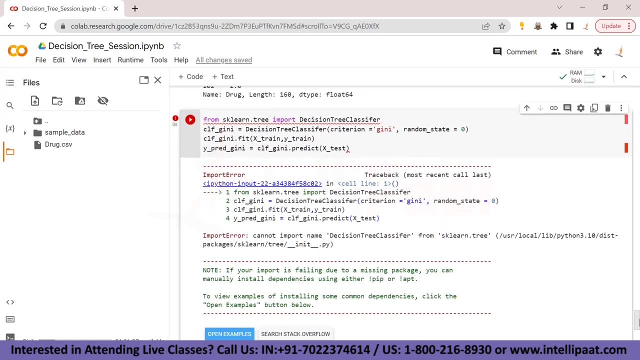 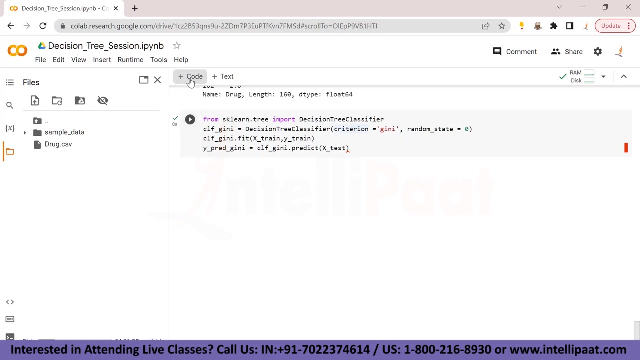 test. now let us run this path of code, alright. ok, so we have made mistake over here in the spelling of classifier, so i will have to add i over here and i over here as well. now let us run this block again. alright, now let us print the prediction. 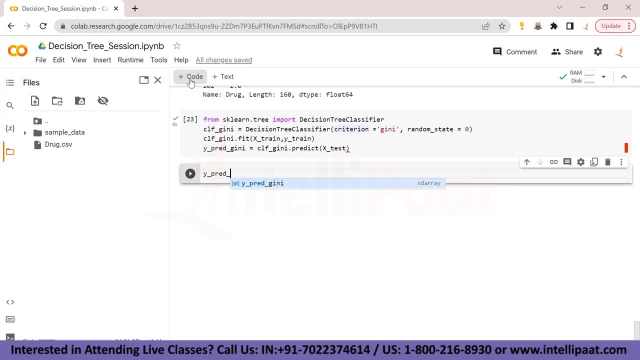 predicted results: y pred underscore gini. so these are the predictions made by our model. alright, now next thing we will do is we will check the accuracy of our model using accuracy underscore score function. so first of all, we will have to load that functionality from sklearn dot matrix. 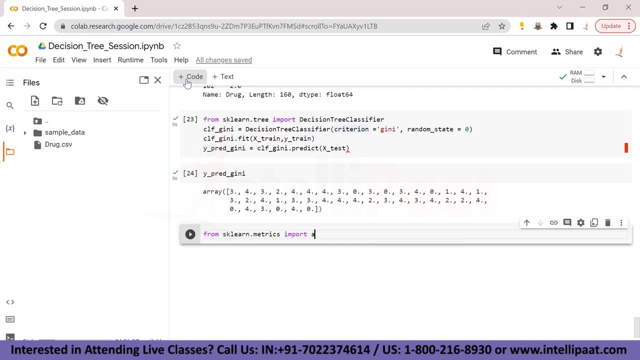 ok, import accuracy underscore score and we will print this accuracy score by making comparison between y underscore, pred underscore, gini and y underscore test, and here you can see that we are getting 100% accuracy. alright, now i hope you guys must be very curious about how decisions were made in the background. 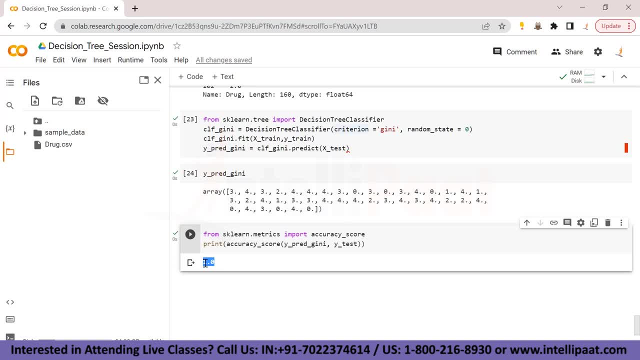 well, i do have a solution to fulfill your curiosity. we will put out a snapshot of background mechanism using the plot of our model and we will use it in the next class. so we will put out a snapshot of background mechanism using the plot of our model and we will put 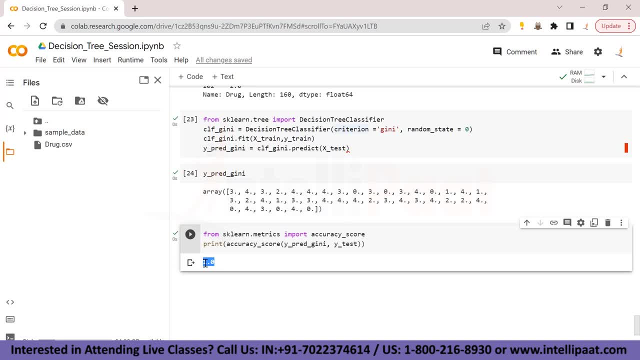 out a snapshot of background mechanism using the plot of our model. and we will put out a snapshot of background mechanism using the plot of our model and we will put out a snapshot. the pattern will be bn 0.6-3- excel here. so we will say, in addition of the tab case, we 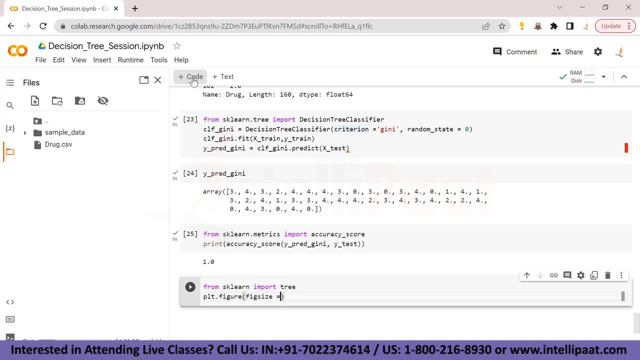 will express the placement, because this is the position of theочки we�� cena conjecture and this is the position gap. so we will do a split inspection of this result and it will only be one touch time from time to time. hence, some total french is started in our Bow, sıkfacts. 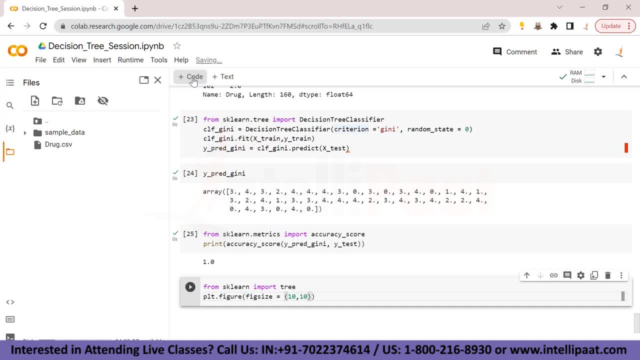 cross 10.. Now we'll use that function that we talked about, that is treeplot underscore tree, and to it we'll pass clf- underscore genie, dot fit, x underscore train, comma y underscore train And finally we'll add the command plt dot show, to represent. 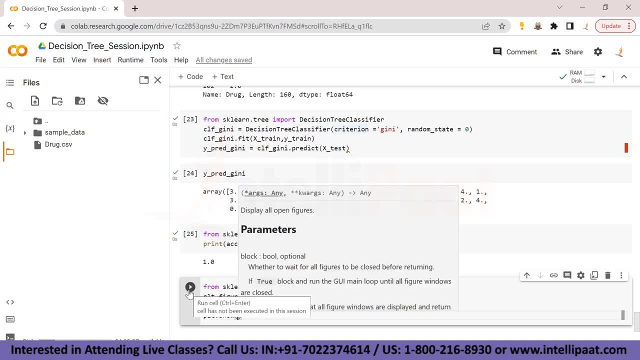 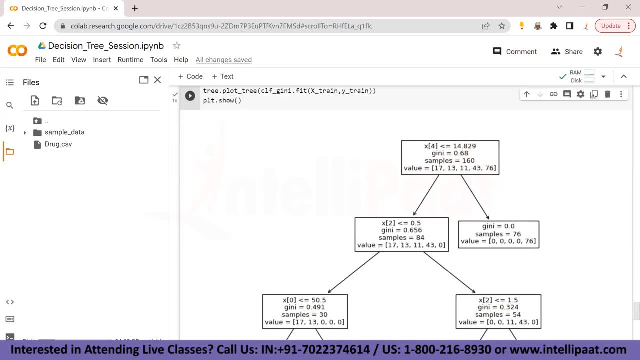 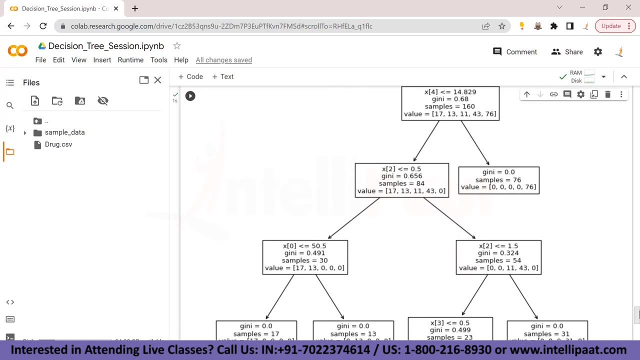 the tree plotting And here you can see how decisions were made based on genie value, And you'll know how each split happens step by step. So this is the best advantage that decision tree offers. After you have created the model, you can visualize the background mechanism that really happened. 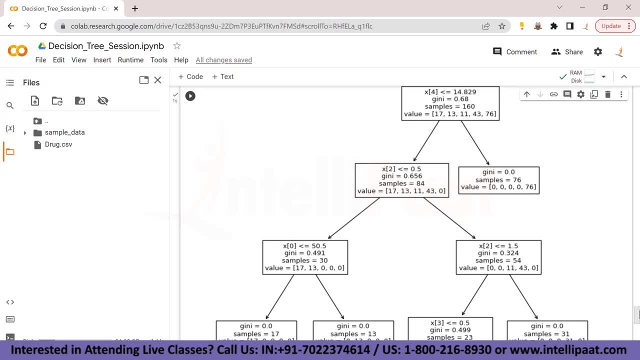 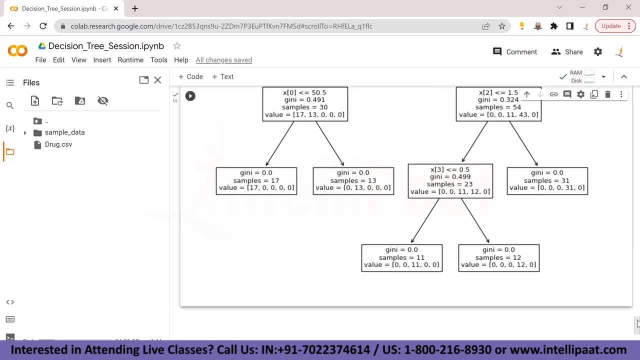 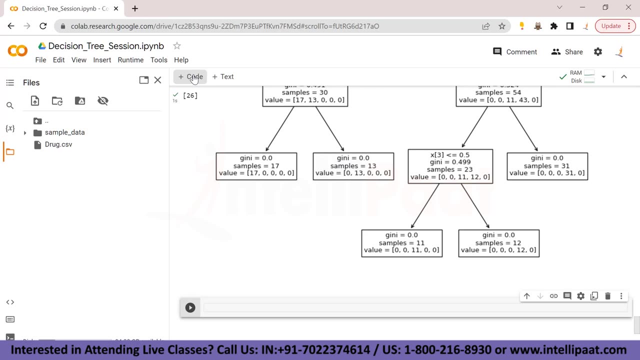 in your machine learning process. All right, Now there are few more parameters that you have with this particular kind of model. You can use different criteria, such as genie, that we have used already. You can use entropy. You can use information gain as well. Let's try what. 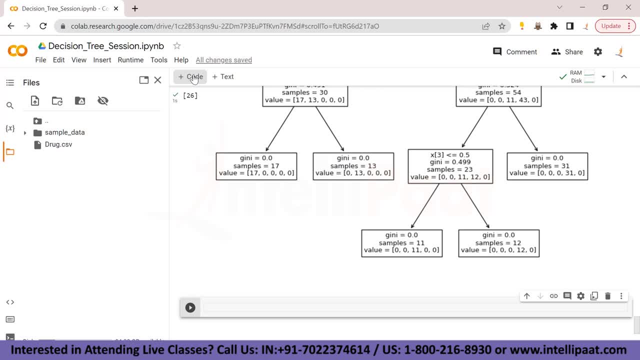 happens with entropy. So for that purpose, let us create a new object, h clf underscore entropy equal to decision tree classifier, and inside it the criteria will be equal to entropy. One more time, One more time, entropy. Now, here we'll introduce one more argument, that is, max underscore depth, which. 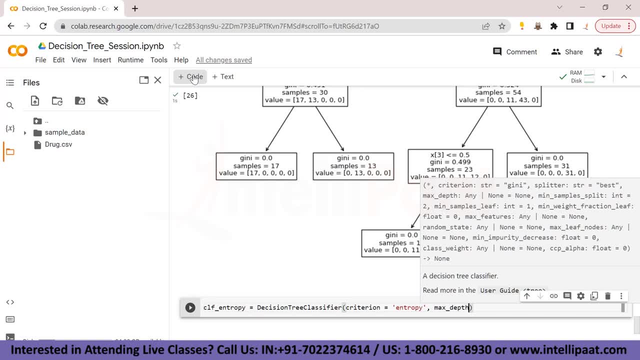 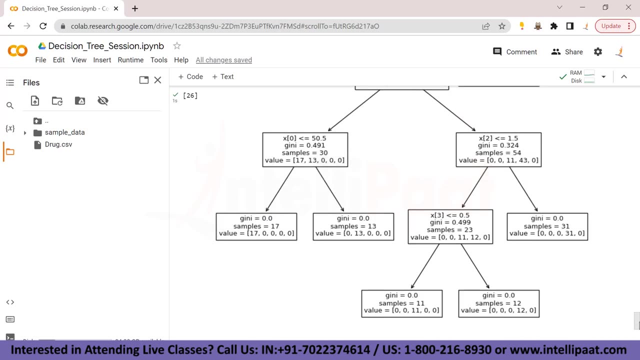 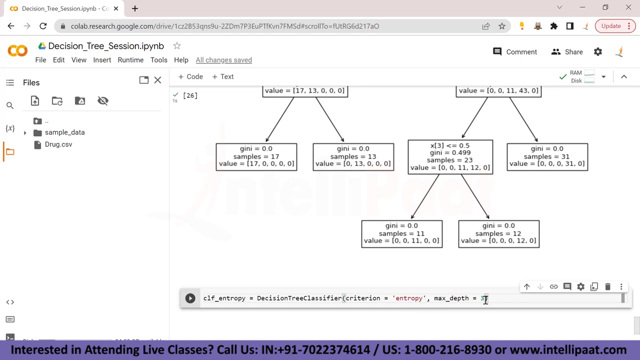 is basically used to control the depth of tree that you want your model to go to. alright, So let us set maxdepth as 3, because in previous layer we have seen that we have 1,, 2,, 3 and 4 layers. So let us see what happens if we set maxdepth as 3. alright, Now we'll set. 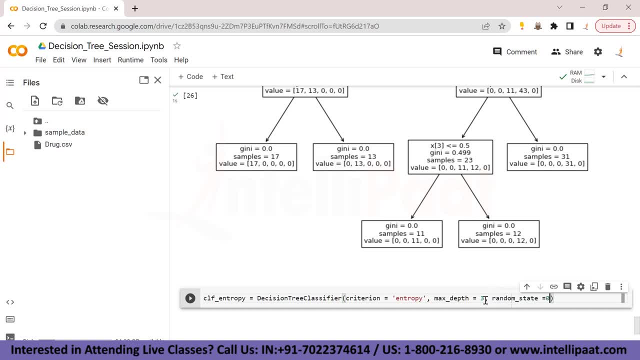 random underscore state as 0 itself. Now we'll fit our data to this particular classifier, that is using entropy as a criteria, And we'll store the predicted results. The variable named as y underscore, pred underscore entropy, And clf- dot underscore entropy, dot predict, x underscore test. 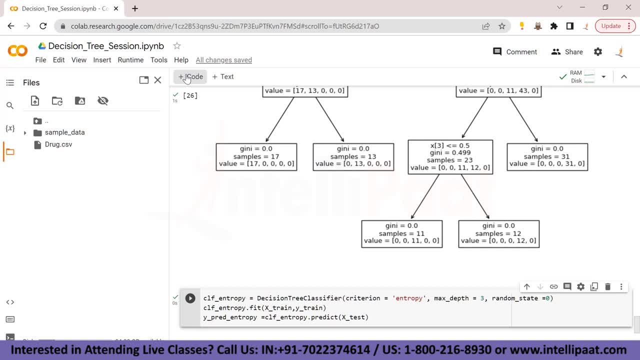 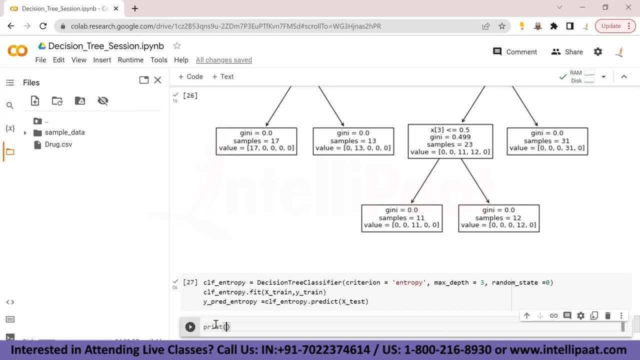 Now we'll run this block And we'll print the accuracy score By comparing y underscore test and y underscore prediction made with the model that has used entropy as a criteria. Alright, Now we'll copy this part of graph that we used previously. 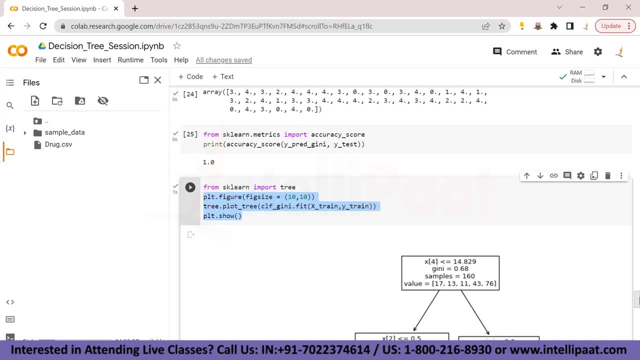 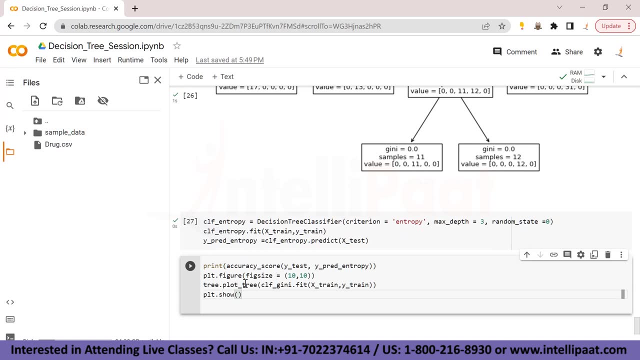 And we'll copy this part of graph that we used previously And we'll print it over here Now. instead of clf underscore genie, We'll use clf underscore entropy over here, And this will show us The graph that has maximum depth equal to 3.. 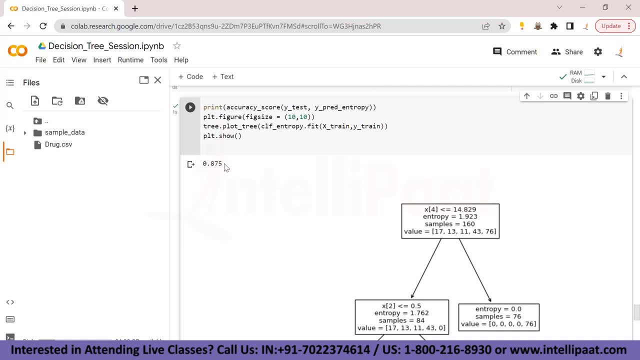 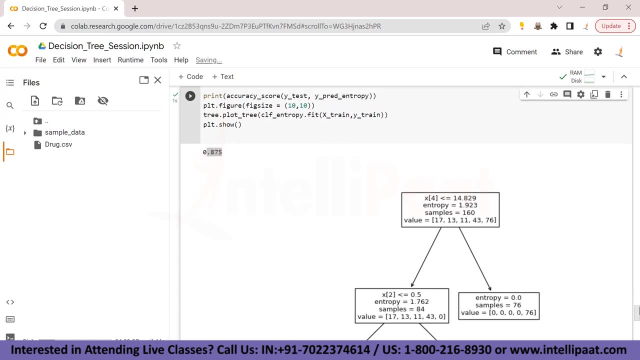 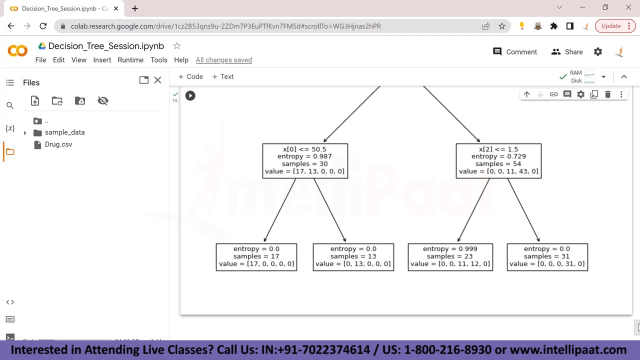 And here you can see that the accuracy has also been reduced because model was unable to classify few samples because its height was pruned with the help of the parameter known as max underscore depth. Alright, I hope now you guys understand the coding implementation of decision tree algorithm with this extensive session.